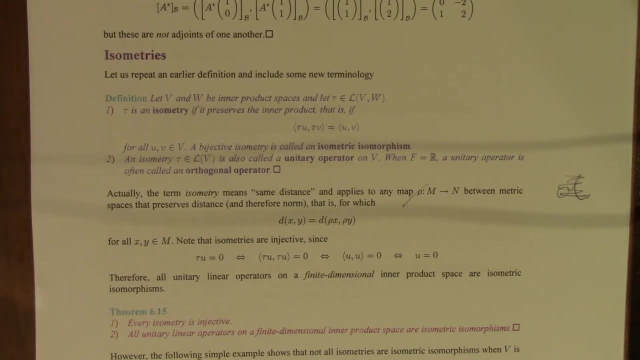 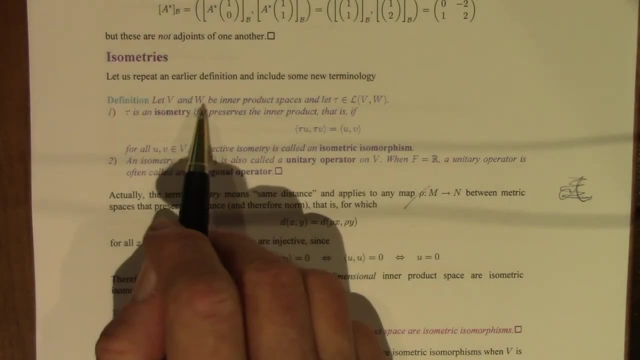 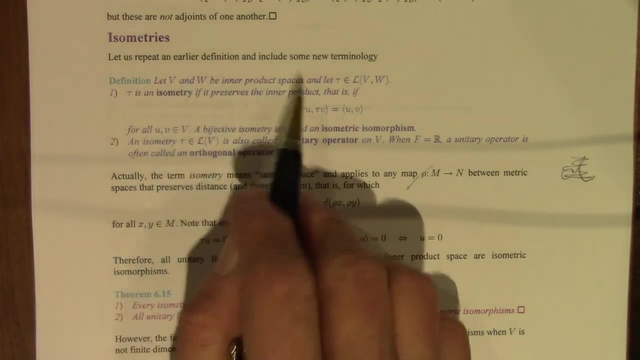 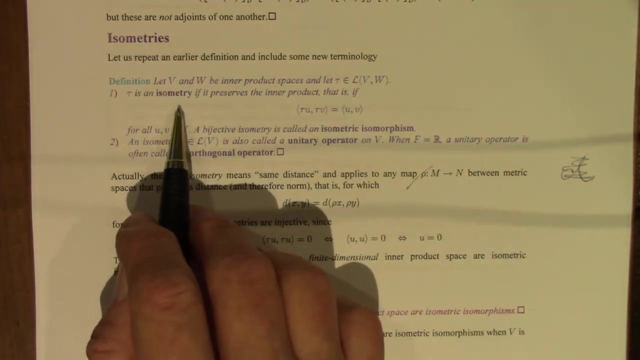 We're going to cover two topics: isometries and the QR factorization. This definition is partially a repeat of an earlier definition. If V and W are inner product spaces and tau is a linear map from V to W, then tau is an isometry if it preserves the inner product. 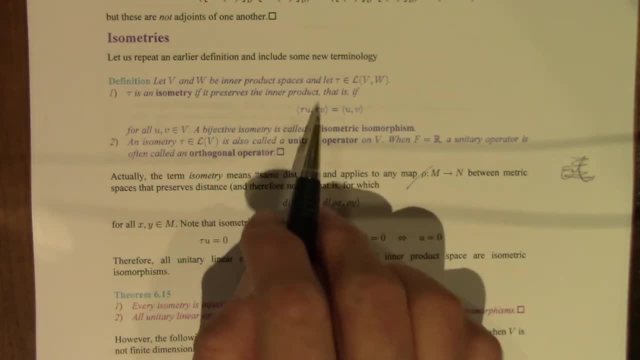 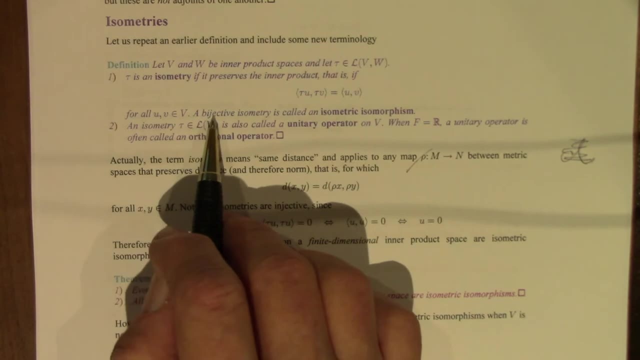 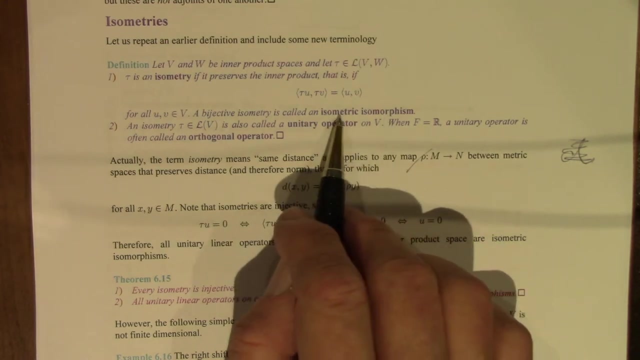 So it looks like this: Tau U inner product, tau V is the same as U inner product V for all vectors U and V. A bijective isometry is called an isometric isomorphism. Isometric is key here because it tells us that the inner product is preserved as well as the algebraic operations. 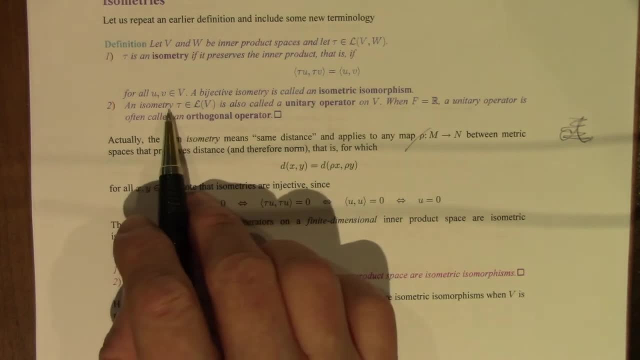 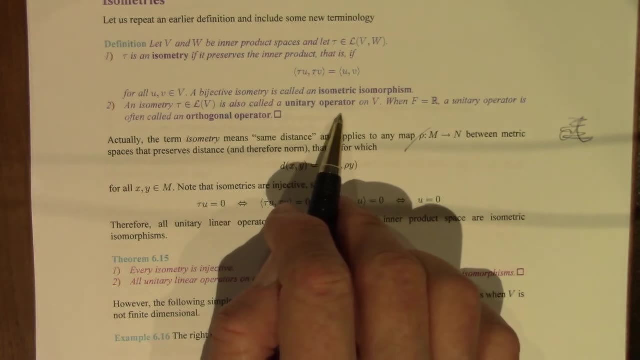 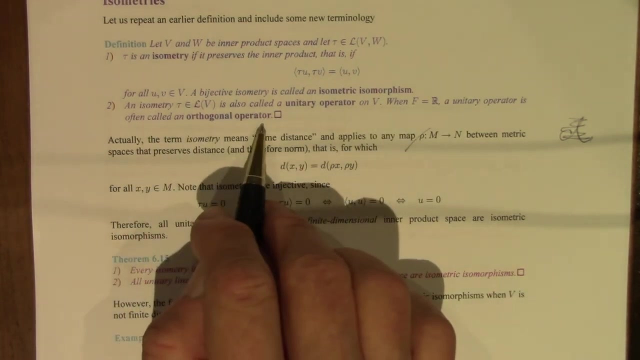 A linear operator on V- V- that's an isometry- is also referred to as a unitary operator, And in the real case this is often called an orthogonal operator. I will probably use the term unitary operator for both cases. 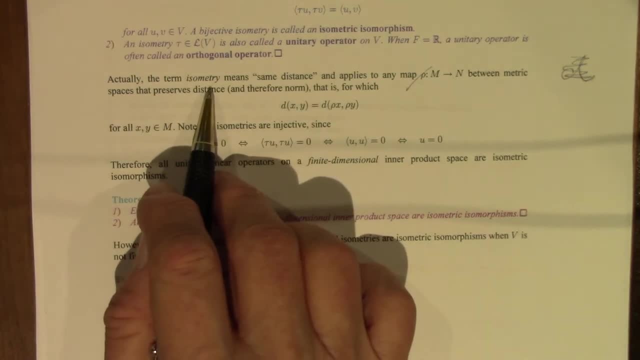 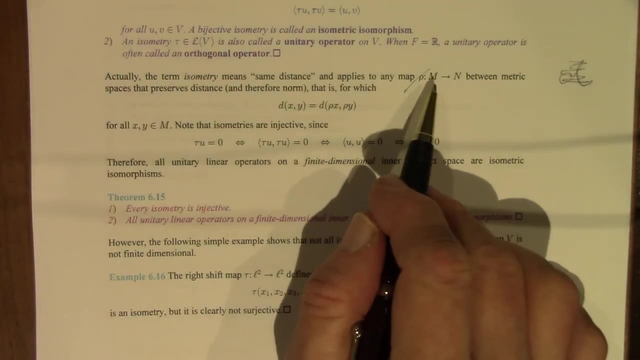 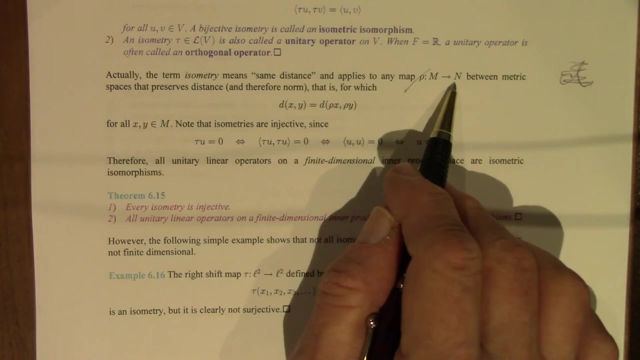 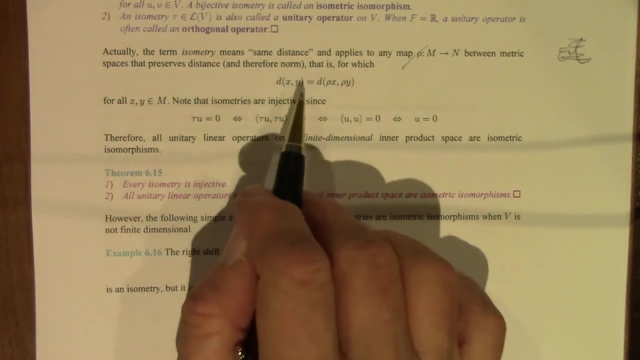 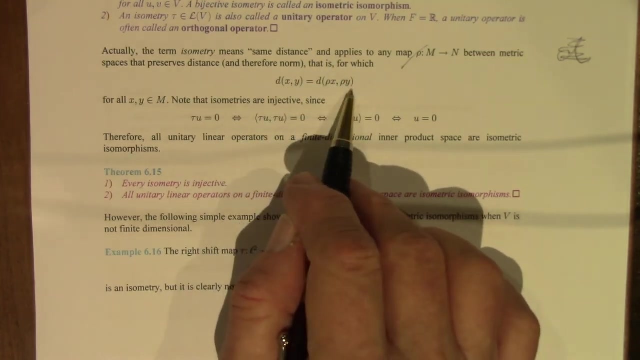 Actually the term isometry, which means same distance, is an unitary operator. The distance applies to any map rho between metric spaces. There doesn't need to be any algebraic structure, just the distance structure, And an isometry preserves that distance and therefore also the norm. so the distance between two elements, x and y, is the same as the distance between rho x and rho y. 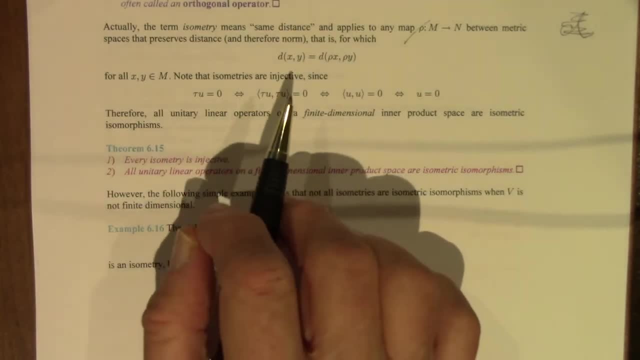 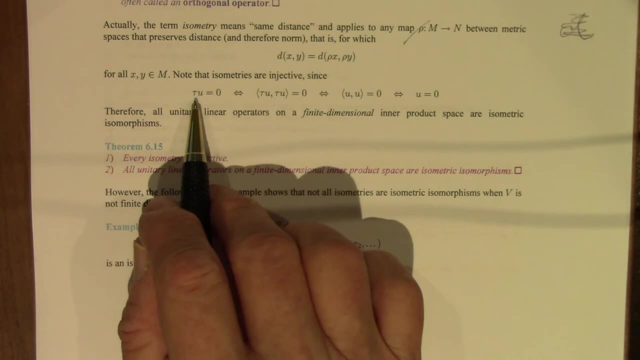 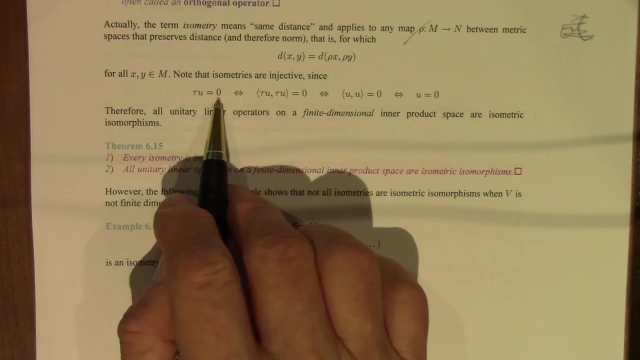 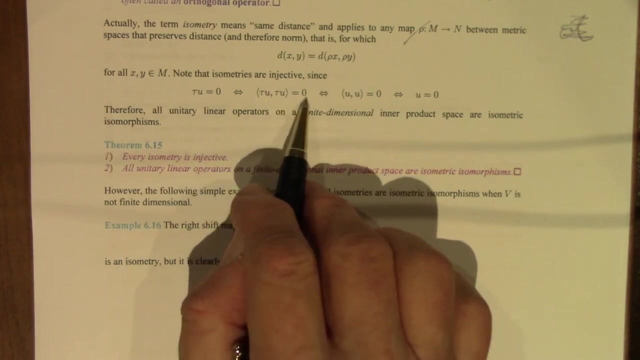 For all x and y, For all x and y. in the metric space, Isometries are always injective. They're linear. so we just have to check the kernel. If tau is an isometry and tau U equals zero, that holds if, and only if, the inner product of tau U with itself is zero. 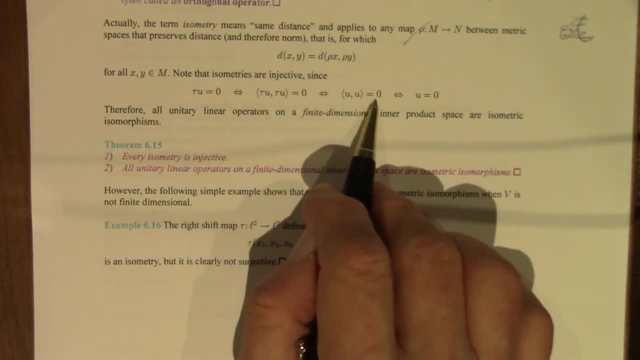 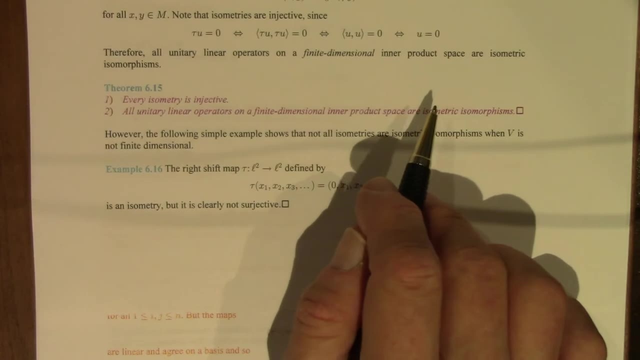 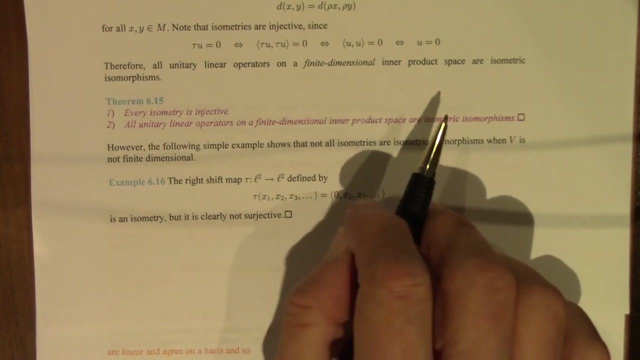 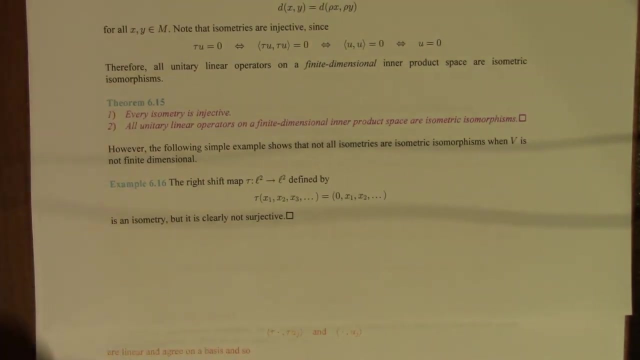 And because tau is an isometry that's equivalent to U- U equals zero, which is equivalent to U equals zero. So the kernel is trivial. This means that all unitary operators on a finite dimensional inner product space are automatically surjective because they're injective. 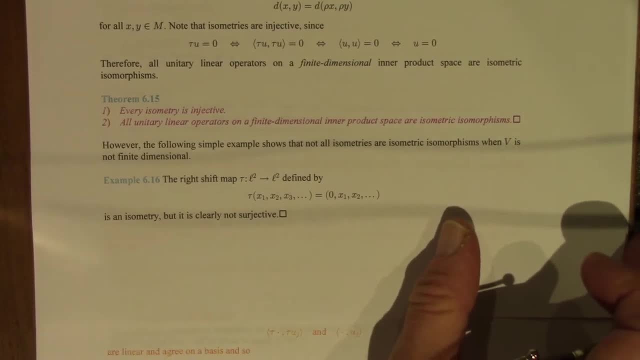 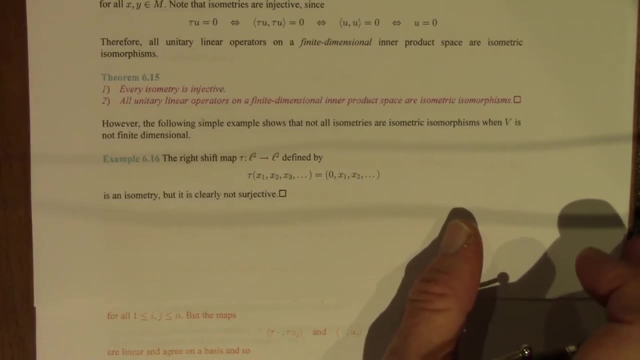 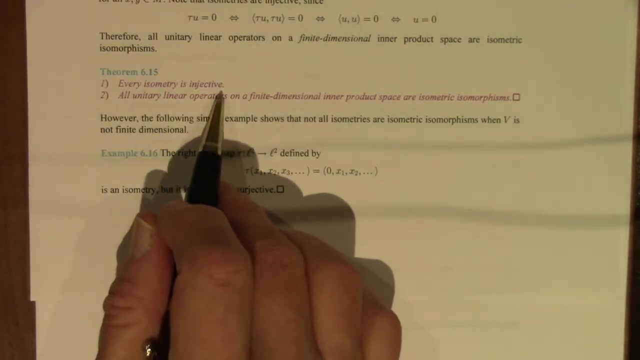 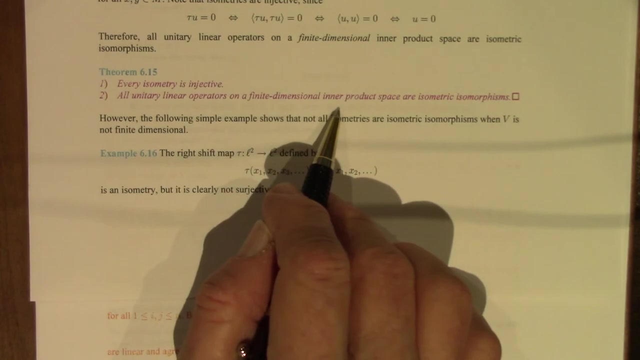 because the dimension of the domain and codomain is the same, It's the same inner product space, And so they are isometric isomorphisms. So, in summary, every isometry is injective. All unitary linear operators on a finite dimensional inner product space are isometric isomorphisms. 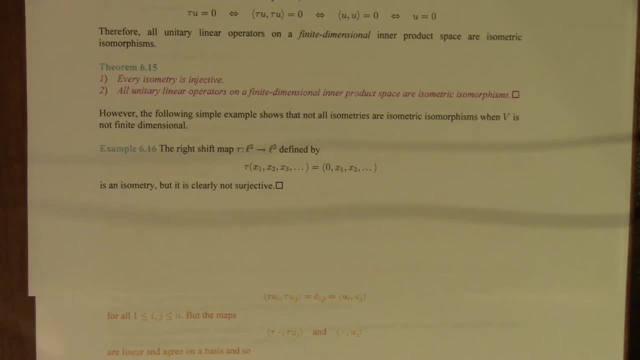 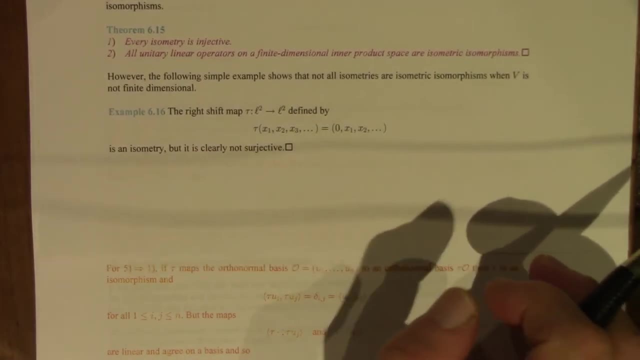 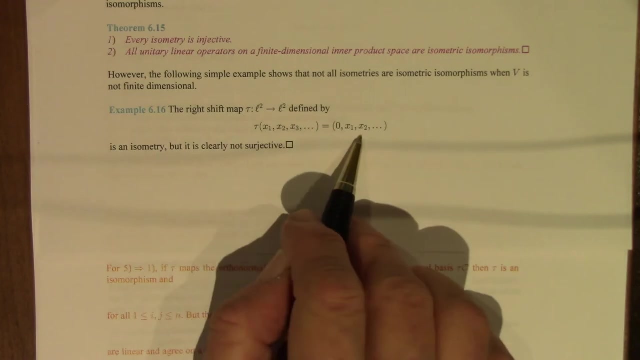 But it's not hard to produce an example that shows that this fails when V is not finite dimensional. The right-shift map on little l2 shifts the sequence one to the right, Every element is shifted one to the right and a zero is placed in front. 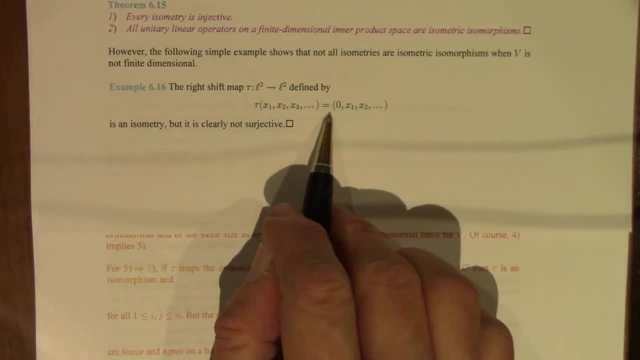 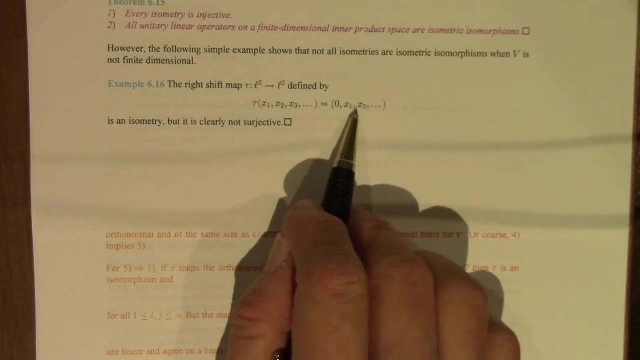 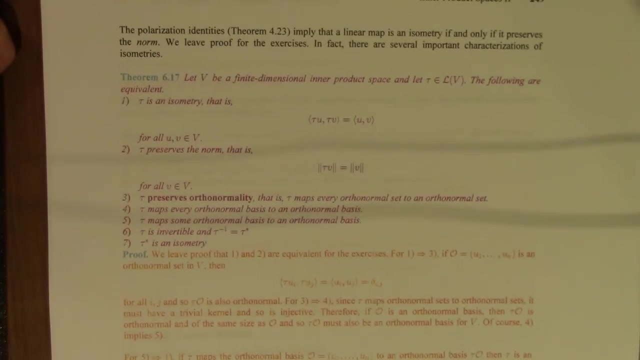 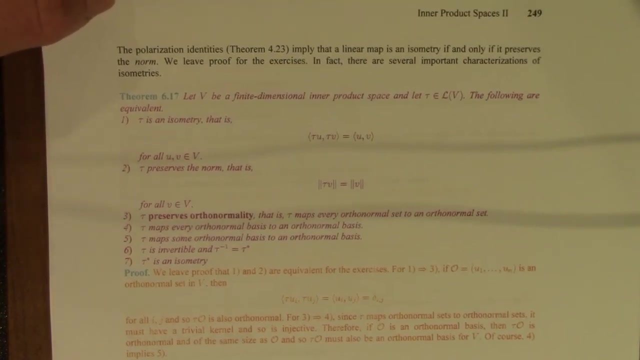 This is an isometry, which I leave you to check, But it's clearly not surjective, So it's not an isometric. isomorphism. Polarization identities imply that a linear map is an isometry if, and only if, it preserves the norm. 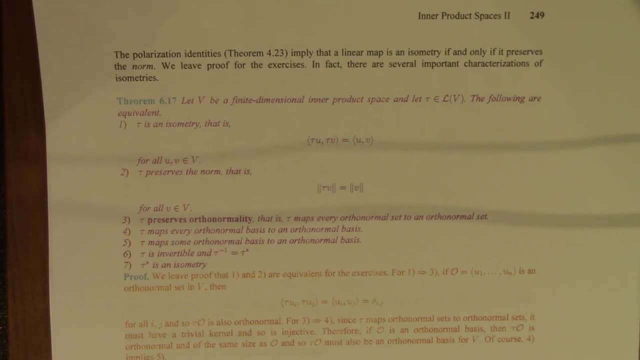 And proof of that is left as an exercise. Proof of that is left as an exercise. This is an important and somewhat surprising. Well, the polarization identities, I guess, are somewhat surprising because they tell us that the norm uniquely determines the inner product. 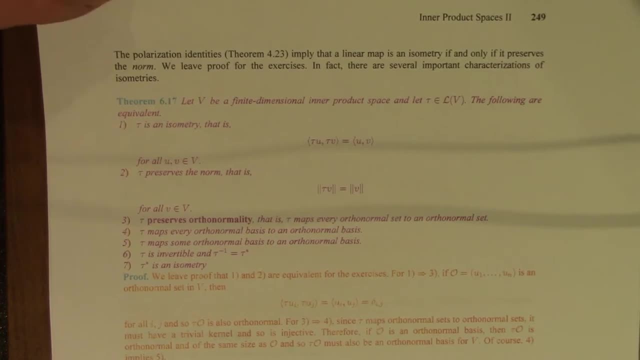 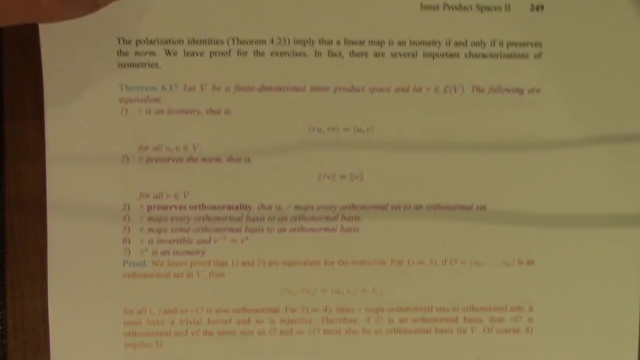 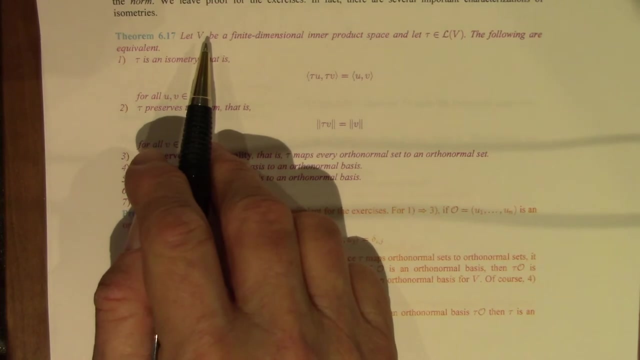 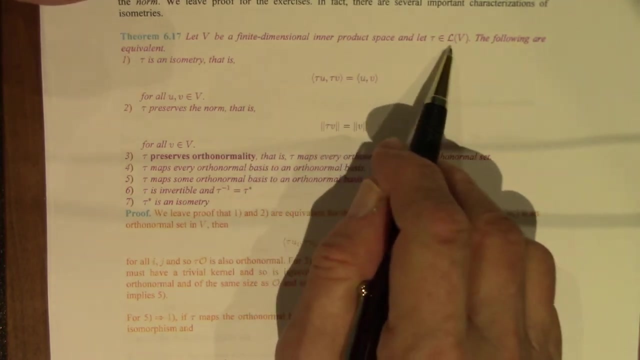 The norm is, in a sense, what seemed to be a weaker concept than the inner product, But it's not. in fact, There are several important characterizations of isometries. Let V be a finite dimensional inner product space and let tau be a linear map on V, linear operator. 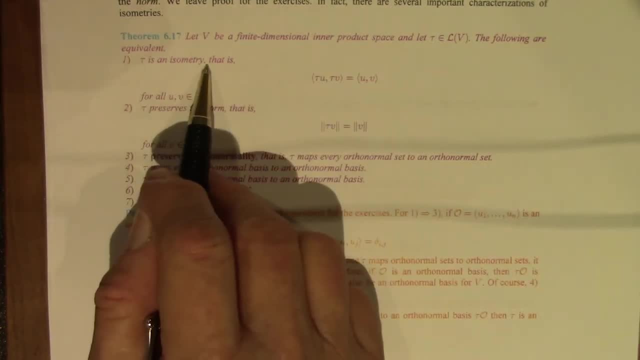 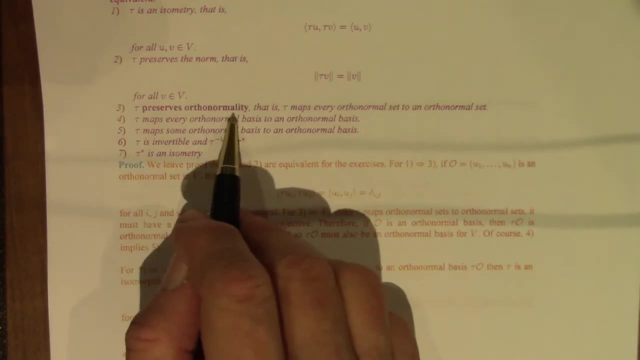 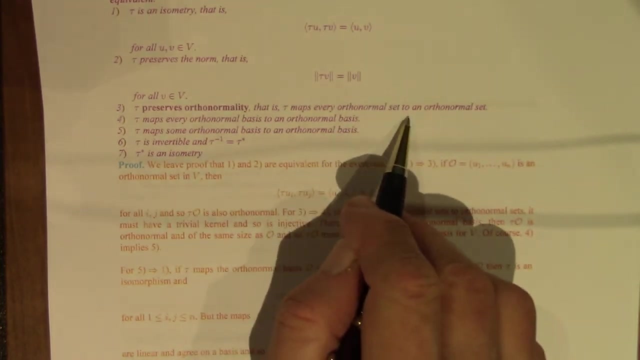 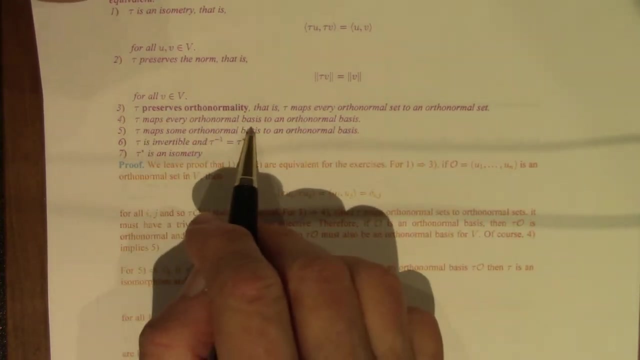 The following are equivalent: Tau is an isometry. Tau preserves the norm. Tau preserves orthonormality. Tau preserves orthonormality, That is to say that tau maps every orthonormal set to an orthonormal set. Tau maps every orthonormal basis to an orthonormal basis. 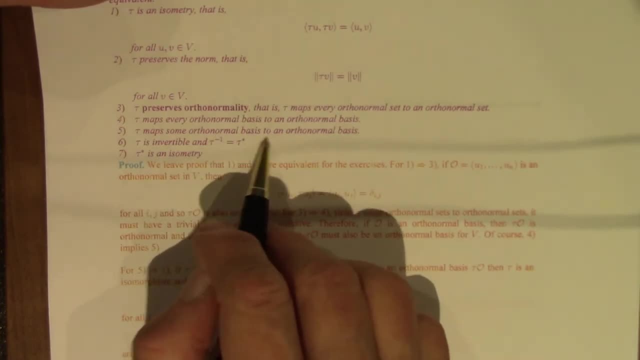 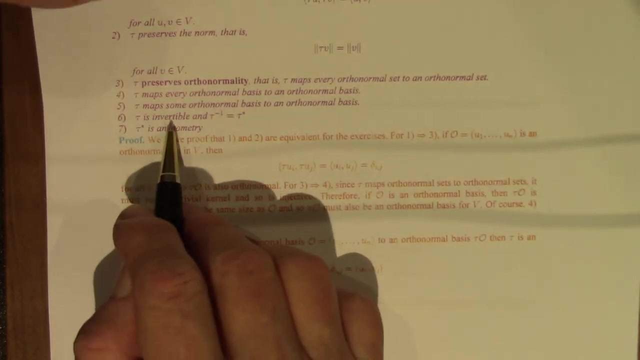 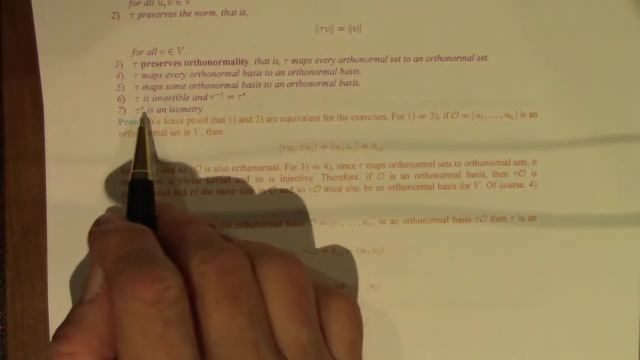 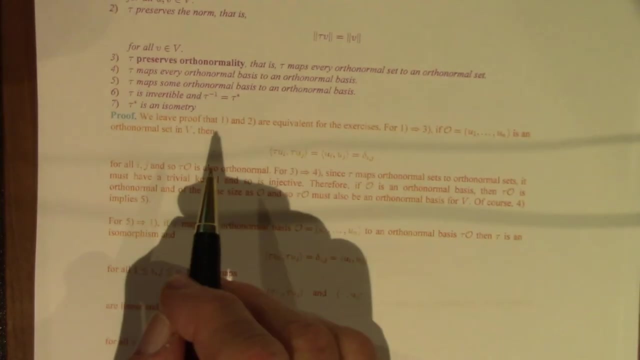 Tau maps some orthonormal basis to an orthonormal basis. Tau is invertible And tau inverse equals tau star, The adjoint of tau. And finally, tau star is an isometry. One and two, the equivalence of one and two. I sort of gave it away. 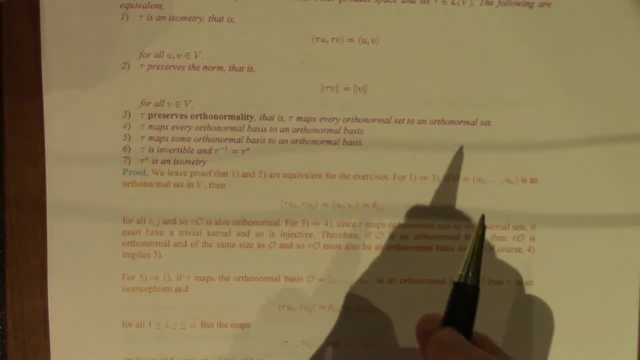 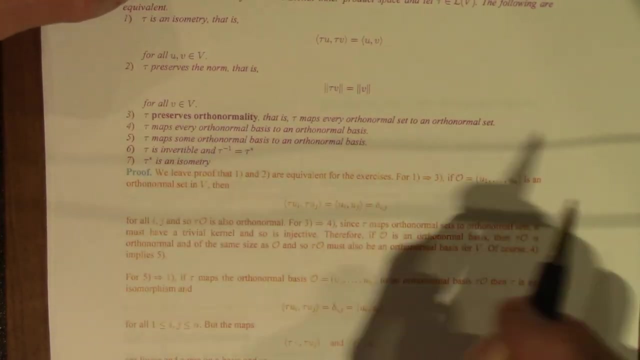 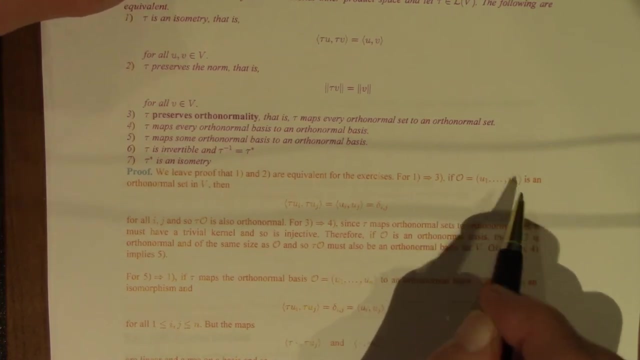 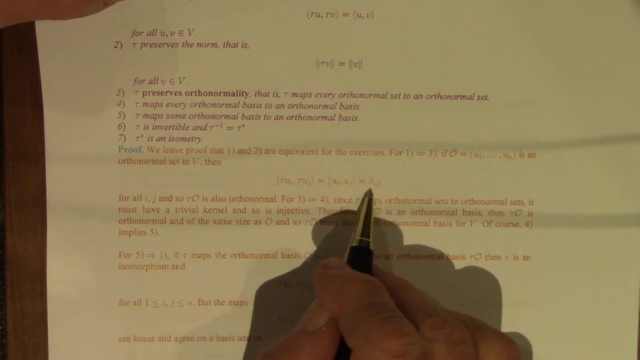 It comes from the polarization identities, So I leave the details to you, For one implies three isometries. preserve orthonormality: If we have an orthonormal set u1 through un, then tau of ui, inner product- tau of uj is the same as uiuj, which is the Kronecker delta ij. 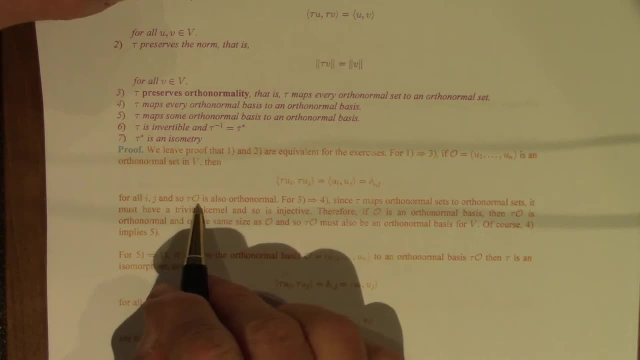 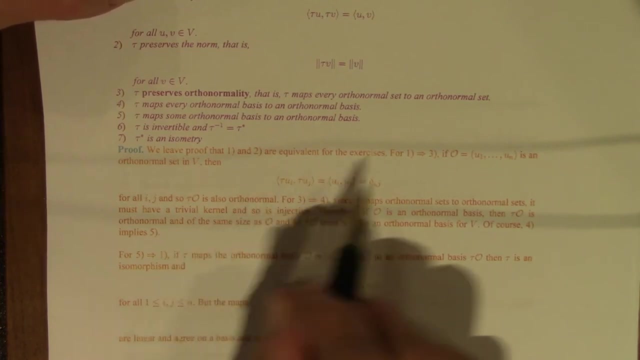 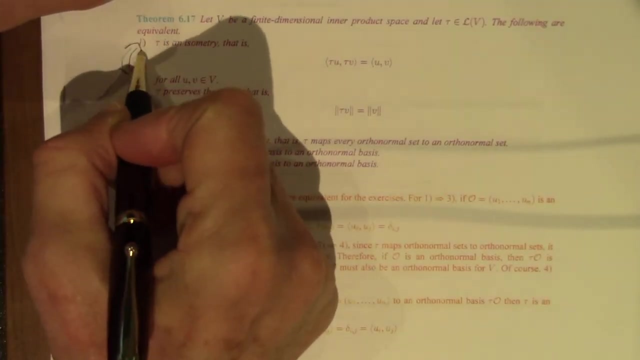 And so the set tau of o- this was the set o- is also orthonormal. So that is one implies three. So far we know, these two are equivalent. Leaving that for u. And they imply whoops, they imply three. 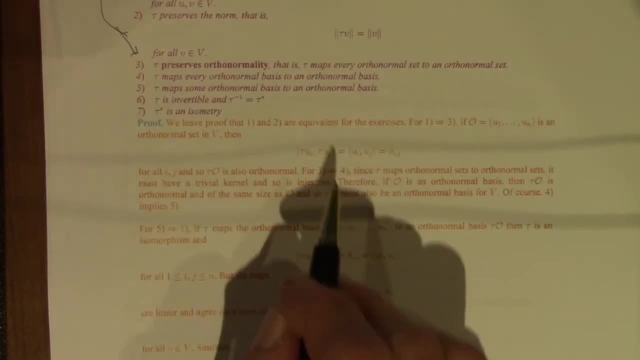 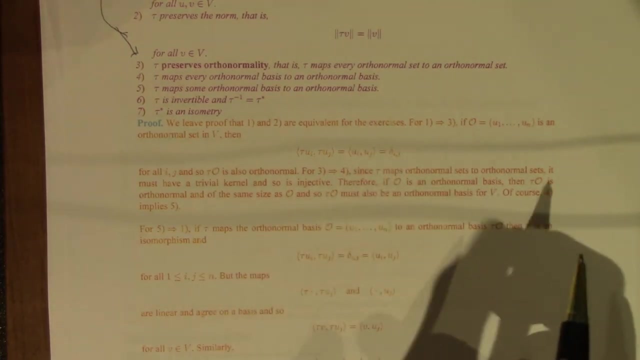 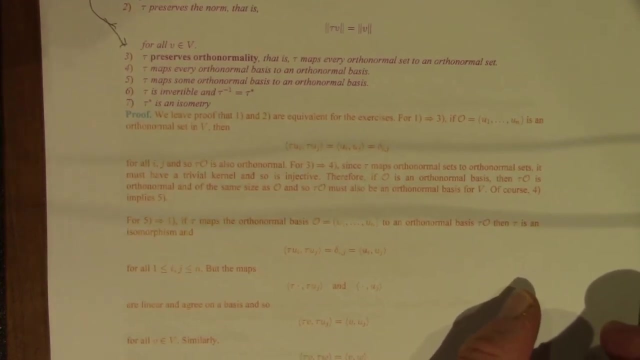 Okay, For three implies four. well, since tau maps orthonormal sets to orthonormal sets, it must have a trivial coefficient, A trivial kernel, And so it is injective. And therefore, if o is an orthonormal basis, then tau of o is not only orthonormal but it has the same size as o. 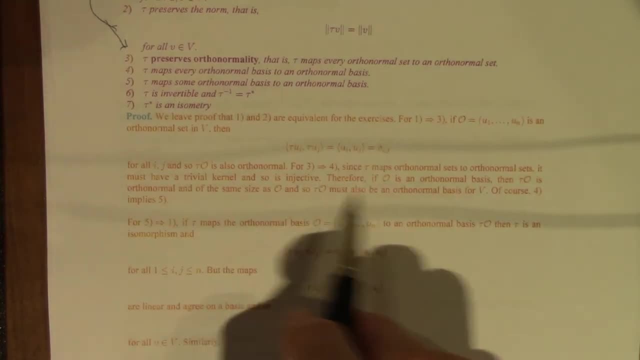 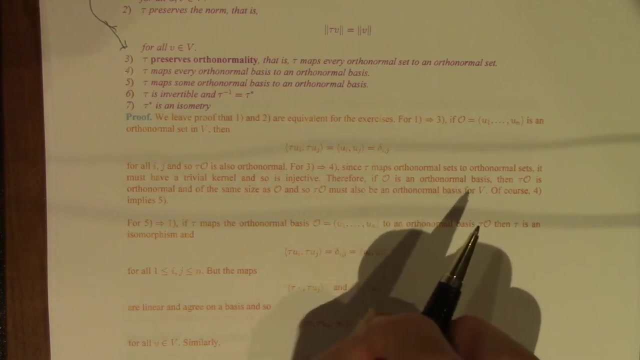 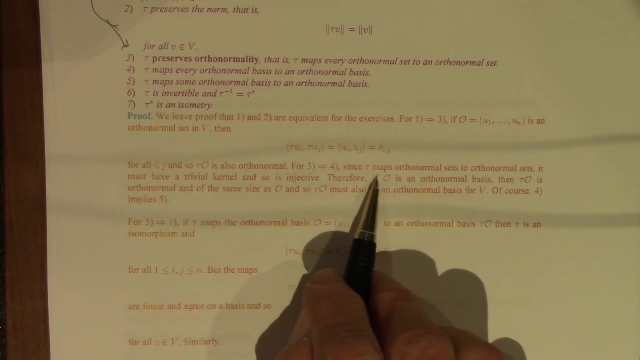 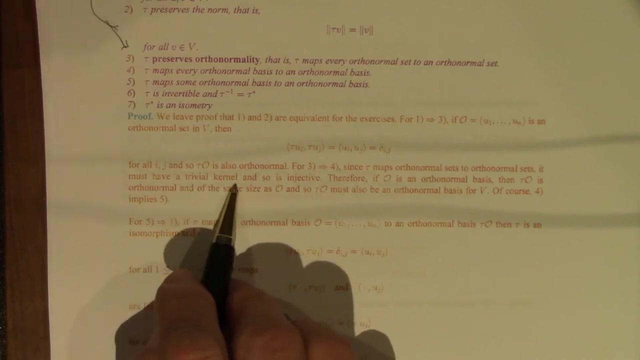 And so tau of o must be, in fact, an orthonormal basis for v. Okay, So what's left here for you to look into a little more carefully is why a map that sends orthonormal sets to orthonormal sets has a trivial kernel. 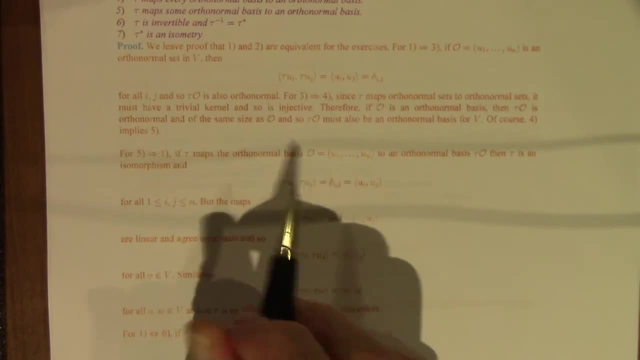 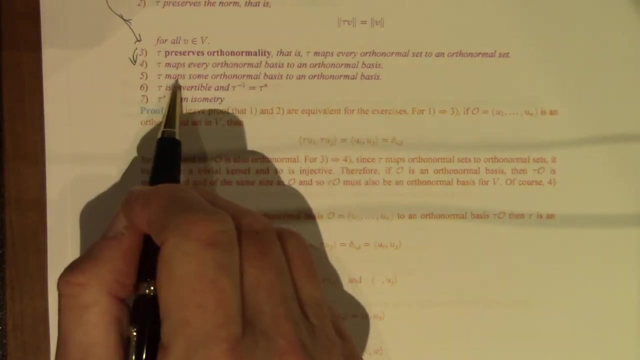 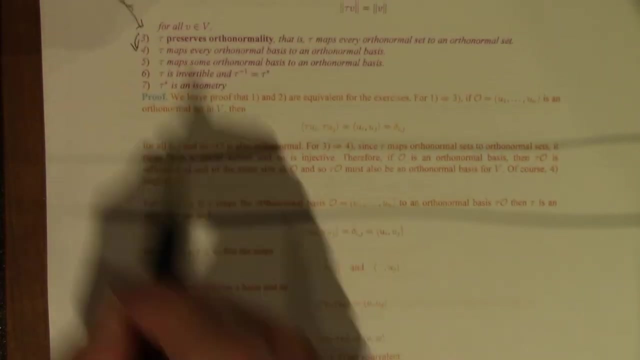 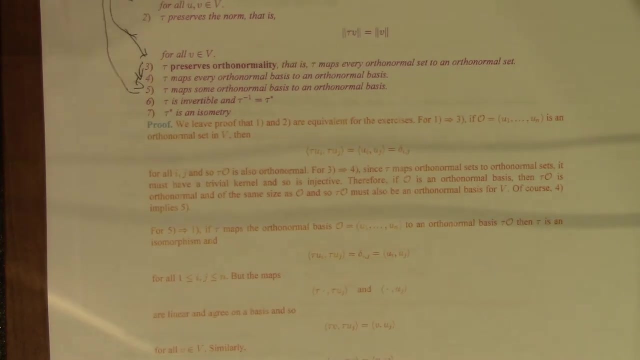 Okay, And of course four. so three implies four. Of course four implies five, Because five is a special case of four And five we can show implies one. So that will tie one through five together. We'll know they're equivalent. 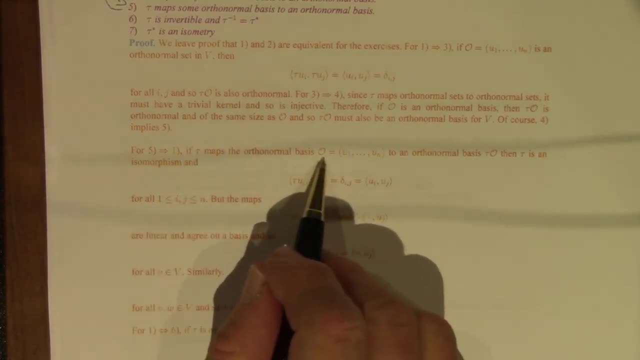 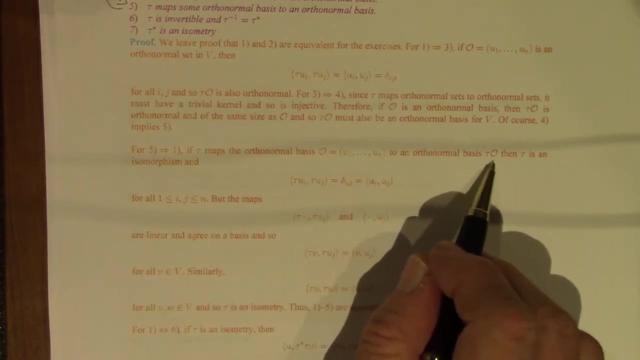 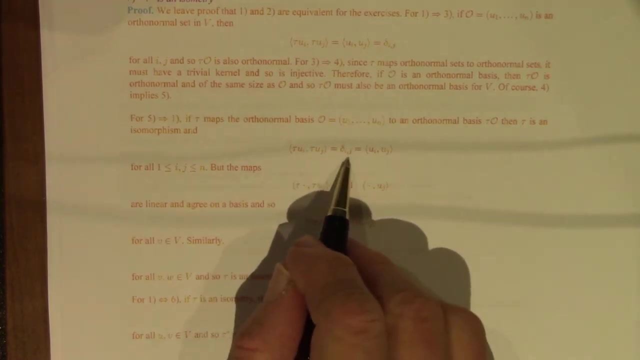 So tau maps an orthonormal basis to another orthonormal basis, tau of o. Okay, So tau is an isomorphism because it maps a basis to a basis. It doesn't matter whether it's orthonormal or not. And tau ui, tau uj is Kronecker delta ij, which is the same as ui uj. 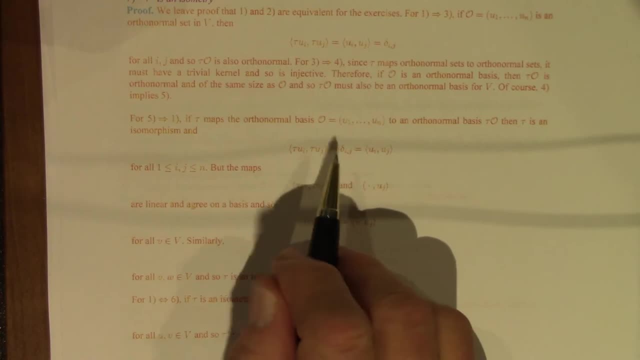 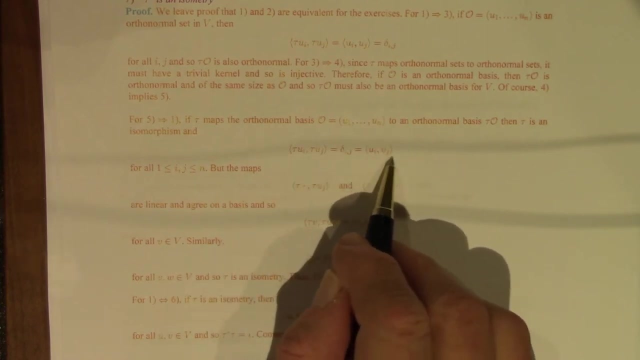 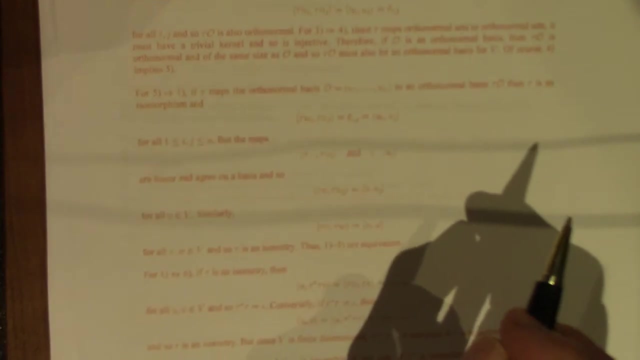 Now we can use the linearity, The linearity in the first coordinate, to upgrade this to tau. of any vector Interproduct, tau of uj is equal to that vector interproduct, uj. Then use conjugate linearity to upgrade the second coordinate. 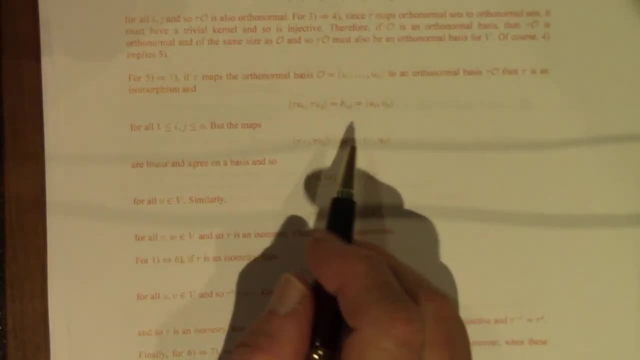 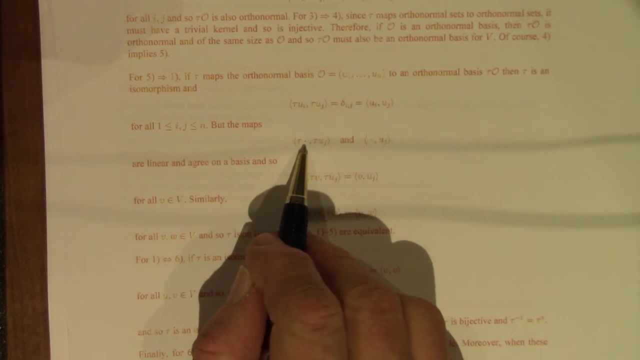 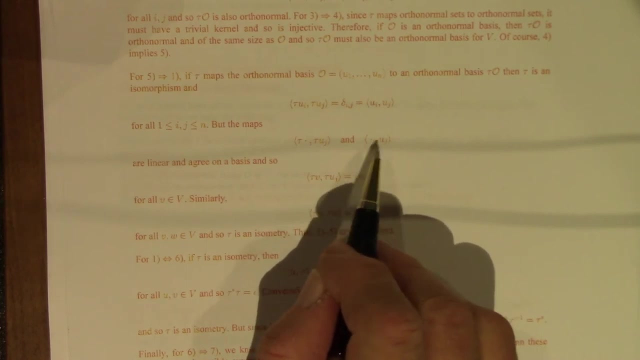 But here's a little bit nicer way to say that This map. I put a dot here. So this is where the variables tau of, say, x, interproduct, tau uj and just x uj, These two maps are linear. 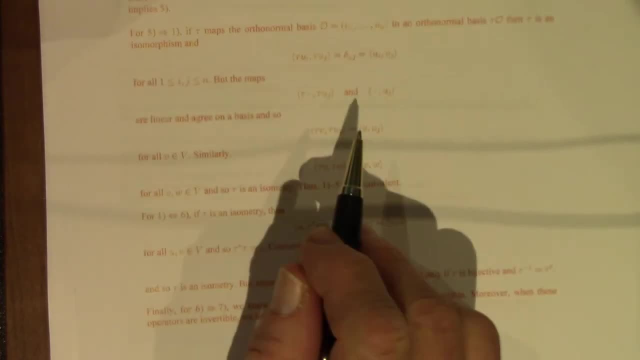 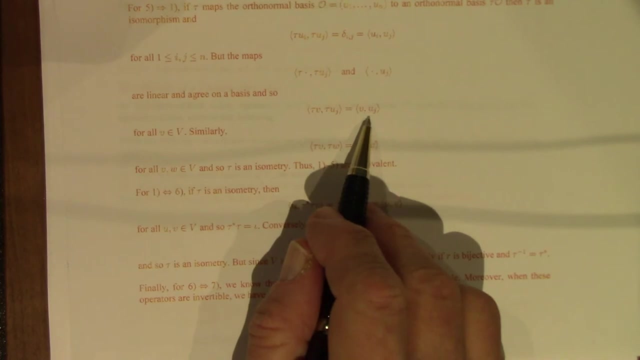 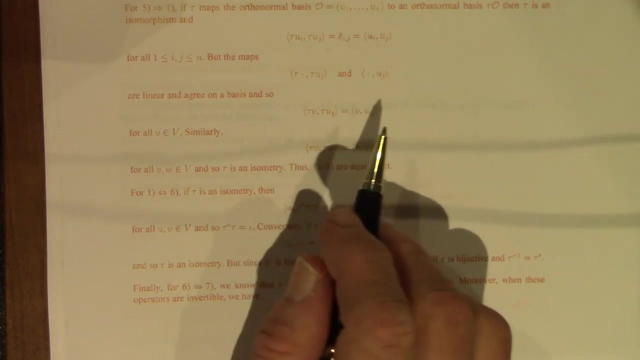 And they agree on a basis. Therefore they agree everywhere. And we can do the same kind of argument. in the second coordinate We have conjugate linearity- Also agree on a basis, And so they agree everywhere. That's something I never proved officially. 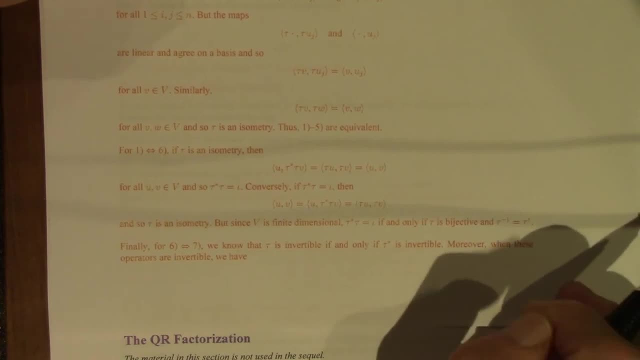 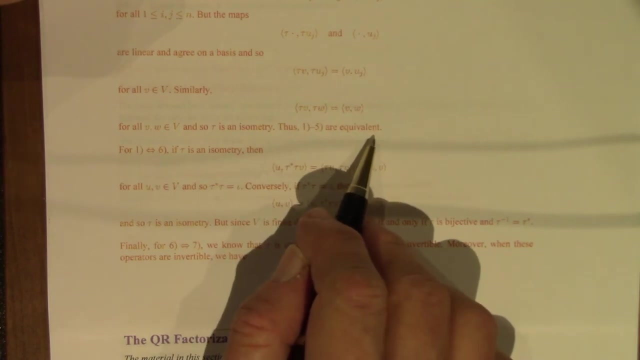 I think I've left that for you, But I will leave it now for you anyway. So 1 through 5 are equivalent Now 1, isometry and 6, invertible. and tau inverse equals tau star If tau is an isometry. 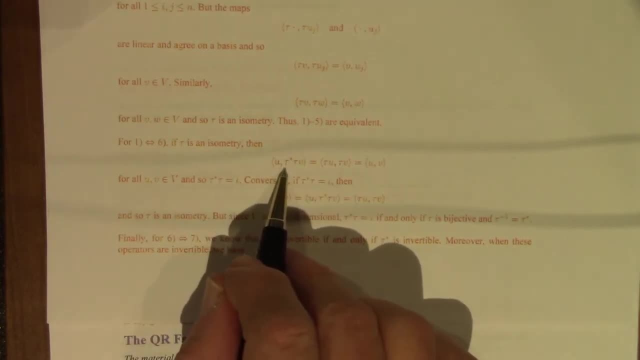 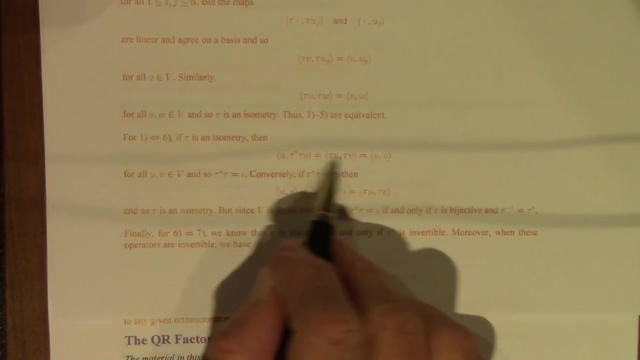 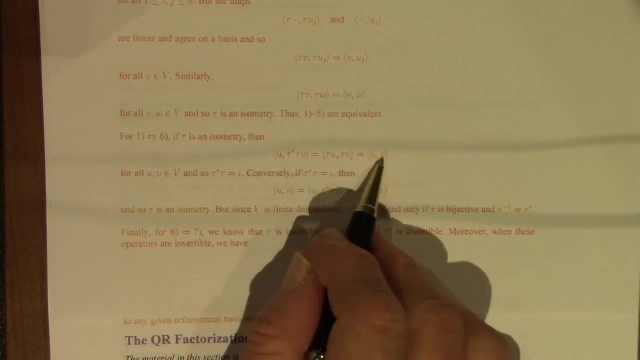 then u. interproduct tau star tau v is tau, u interproduct tau v, which is the same as interproduct uv, And so this tells us that we had a theorem earlier that these two operators are the same. This is the identity. 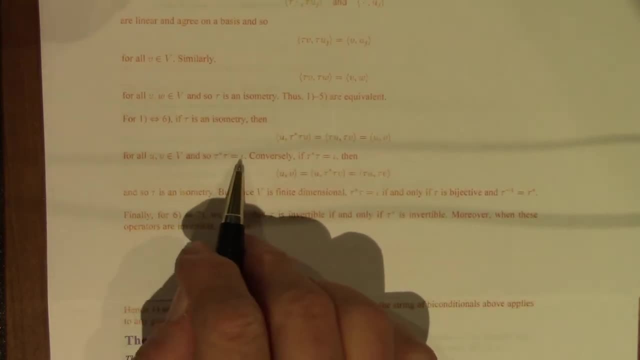 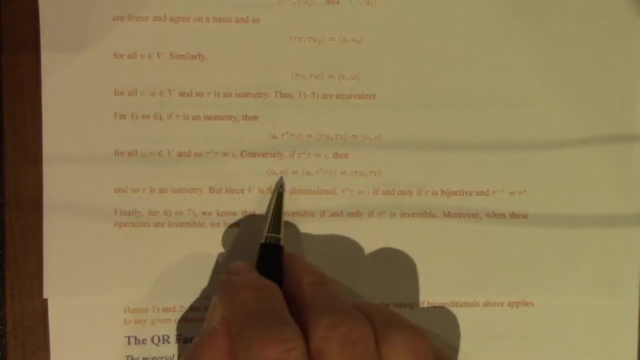 So tau star, tau is the identity And since the operators are invertible, it tells us that tau inverse equals tau star, And that's something you should write out, probably explain in a little more detail. Conversely, if tau star, tau equals the identity, 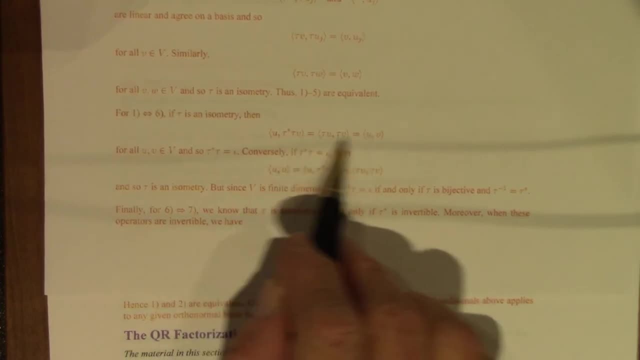 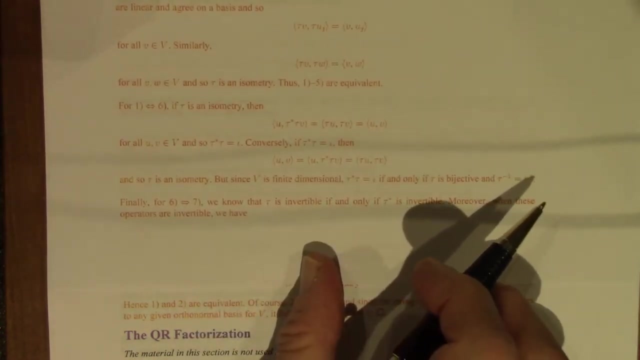 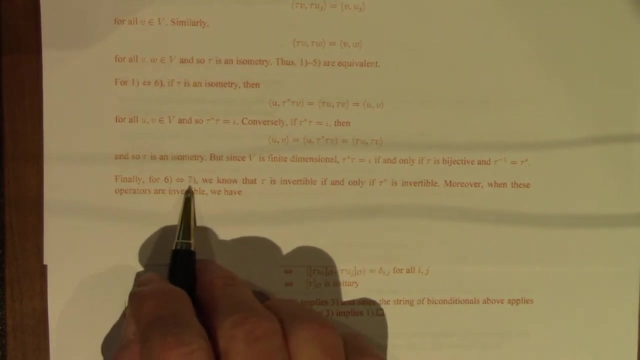 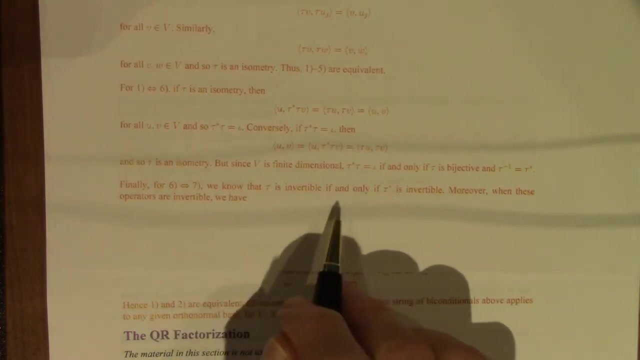 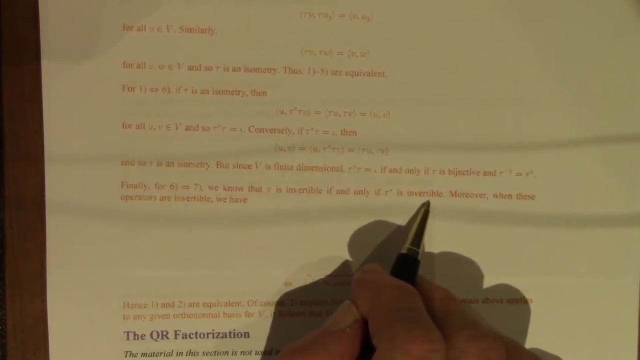 then we have this string, which is a permutation of these, Which tells us that tau is an isometry. Finally, 6 and 7 are equivalent. We know that tau is invertible if, and only if, tau star is invertible, And that's something that follows from. 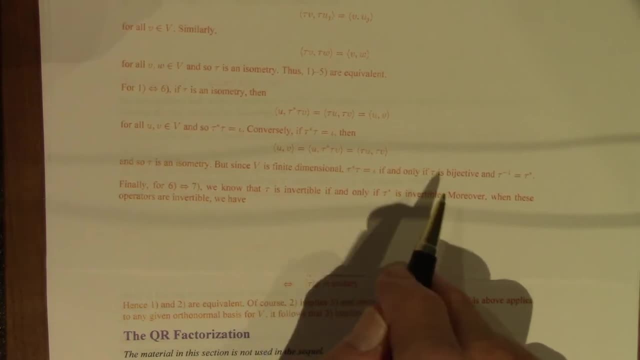 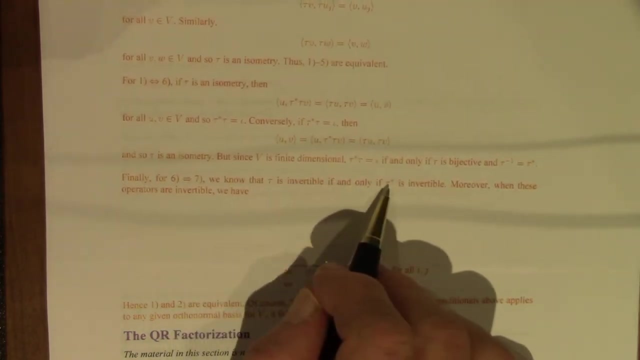 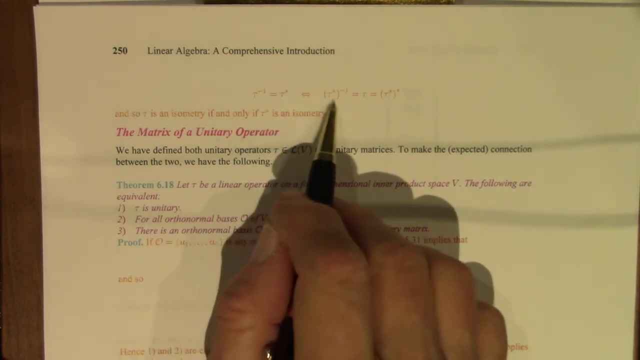 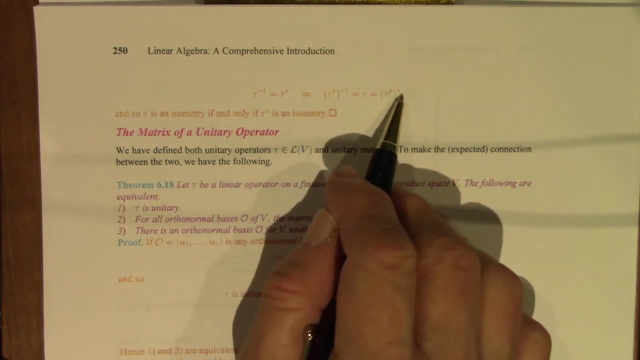 an earlier theorem or corollary, I don't remember which, in this chapter And when these operators are invertible, we have: tau inverse equals tau star, if, and only if, tau star inverse equals tau equals tau star star. Okay, So what we did was we applied. 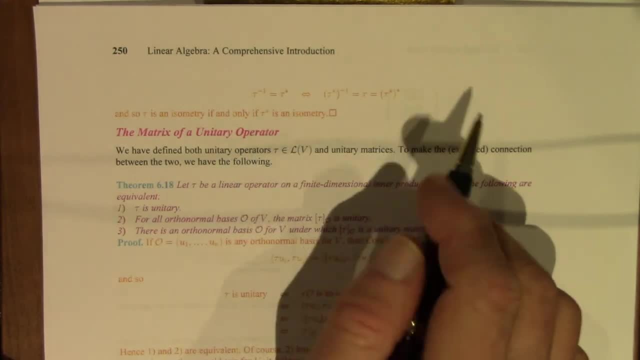 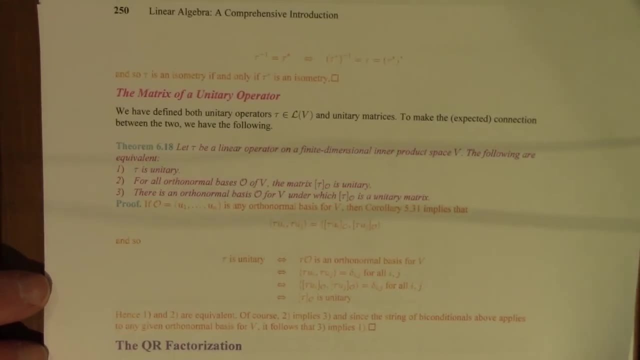 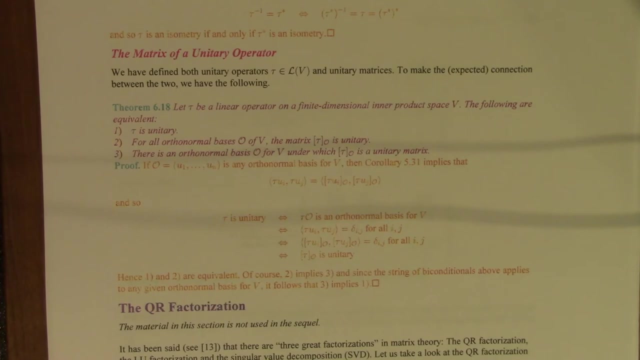 the adjoint here in each direction. So tau is an isometry if, and only if, tau star is an isometry. Now what about the matrix of a unitary operator? What can we say about it? There must be something special about matrix representations for unitary operators. 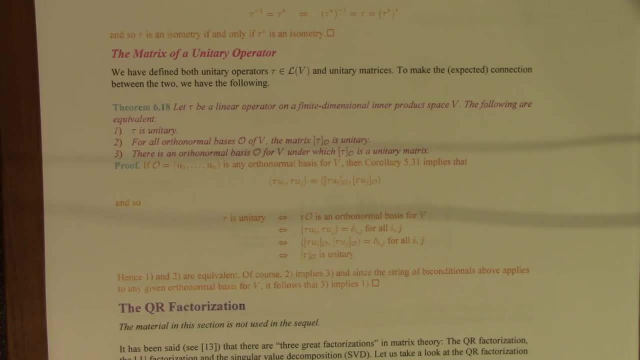 because unitary operators are special. We have defined earlier the notion of a unitary matrix. If you recall, it's a matrix whose columns are orthonormal or equivalently, the rows are orthonormal or equivalently. tau is invertible. 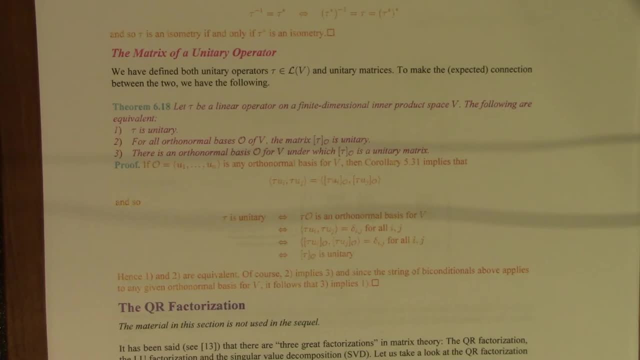 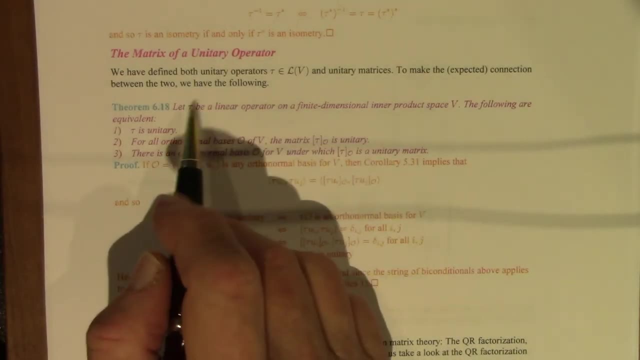 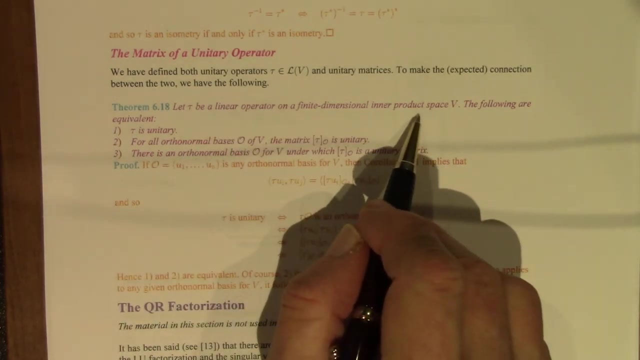 and its inverse is equal to its adjoint, Just like we same thing that we just proved for operators. Here's the connection. Tau is a linear operator on a finite dimensional interproduct space. The following are equivalent: Tau is a unitary operator. 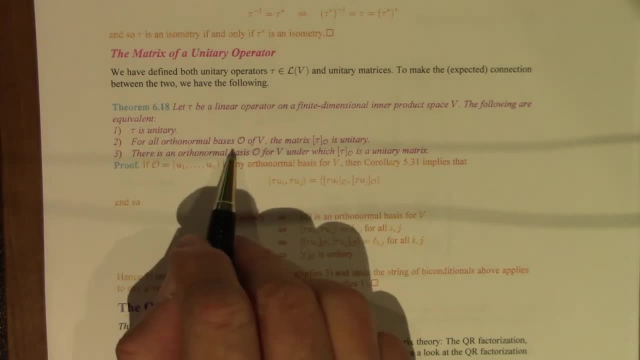 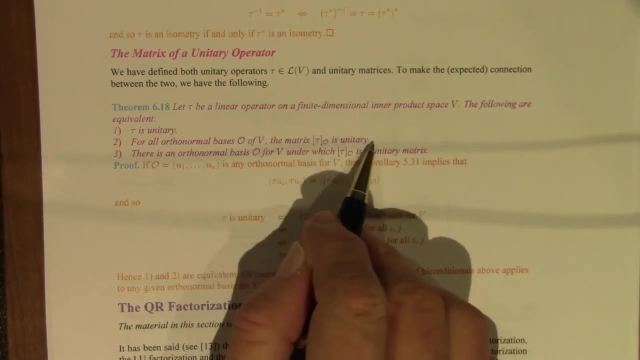 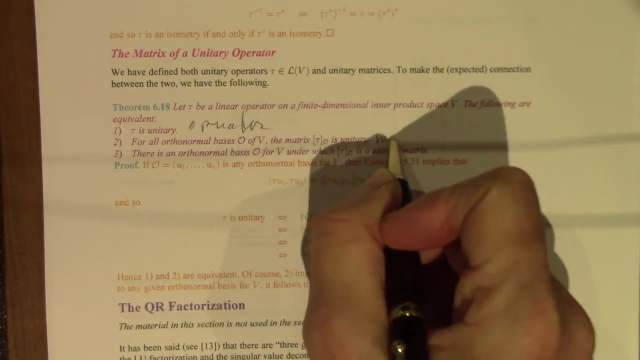 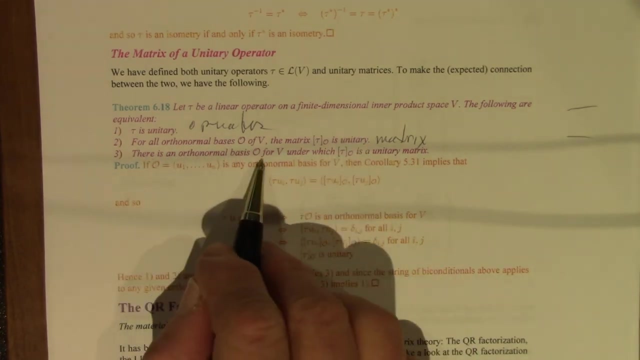 for all orthonormal bases O. The matrix representation of tau with respect to O is a unitary matrix. Maybe I should add those words operator matrix, just so we just to avoid any confusion. There is an orthonormal basis O. 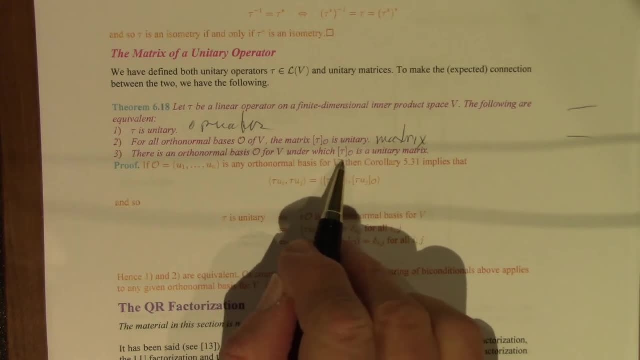 under which the matrix representation of tau is a unitary matrix. I'm not going to go through the proof because I'd like you to think that when you think about it it will be good practice. I think Basically follows from the definitions. 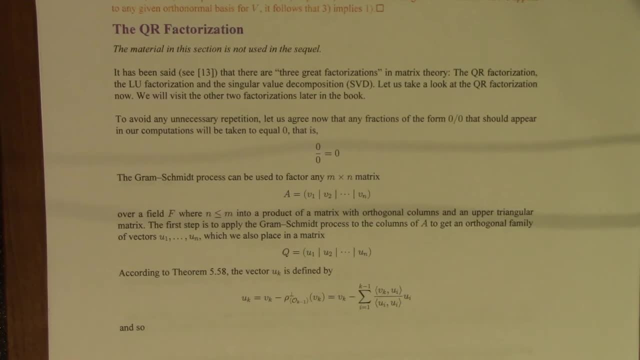 Now let's talk about the QR factorization of a matrix. This material, as I mention here in the book, is not going to be used in the sequel, but it is important, It has been said and I gave a reference in the book. 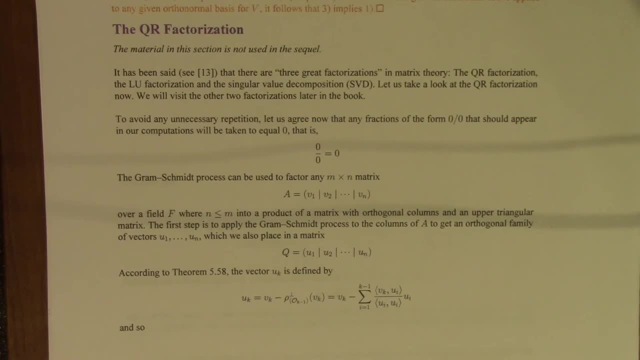 to a very important book on linear algebra, a very important author. It has been said by this author that there are three great factorizations in matrix theory. These are his words. One is the QR factorization, one is the LU factorization. 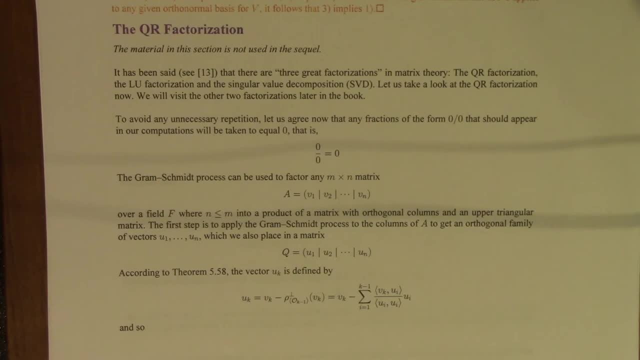 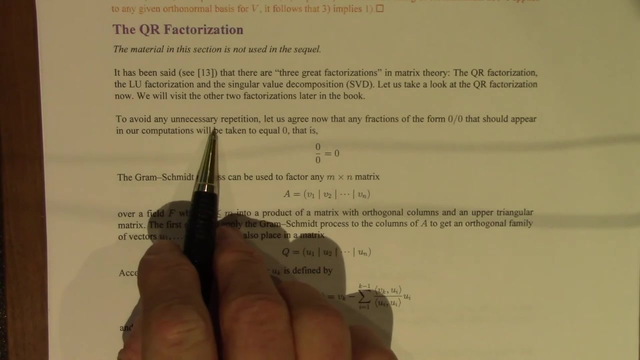 and one is the singular value decomposition. So we'll look at the QR factorization now and we'll visit the other two factorizations later in the book. My recollection is that I left them for topics, chapters, To begin with, just a technical detail. 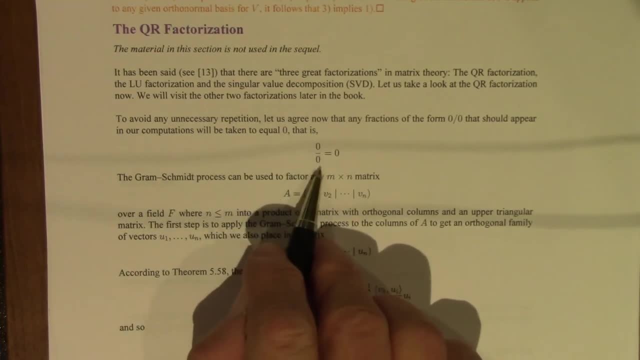 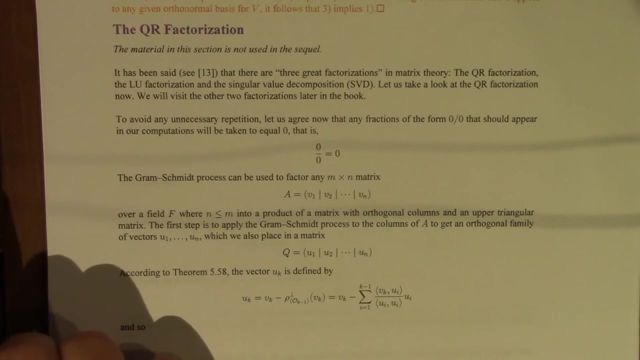 these quotients- 0 over 0, are going to possibly come up in our computation, So we're going to agree now that this is always equal to 0. It's simpler than having to say if the quotient is 0 over 0,. 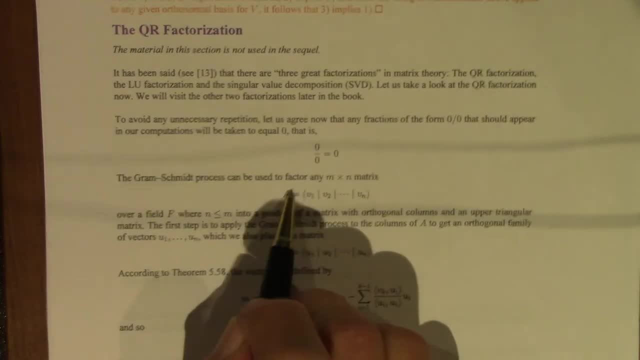 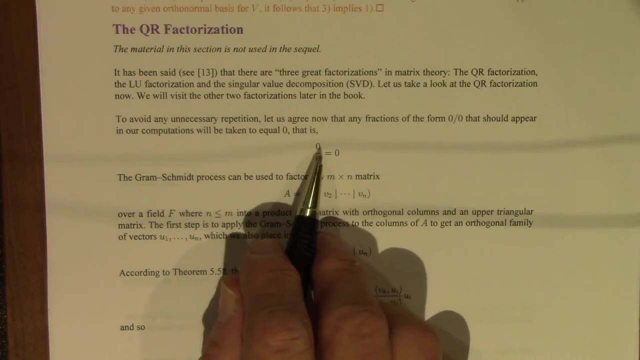 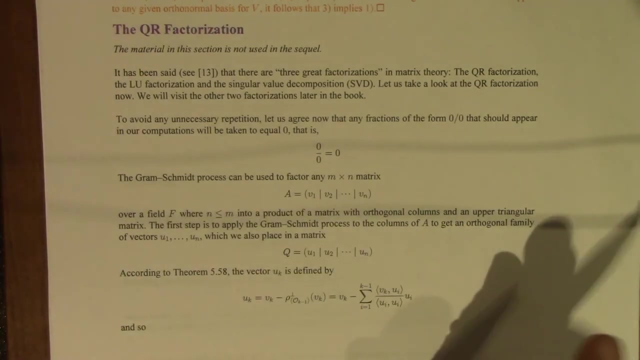 then ignore it. So this is an expedient expedience, more than anything else, and it's temporary. I certainly wouldn't claim that everyone thinks 0 over 0 is equal to 0. Most people would simply say it's undefined. 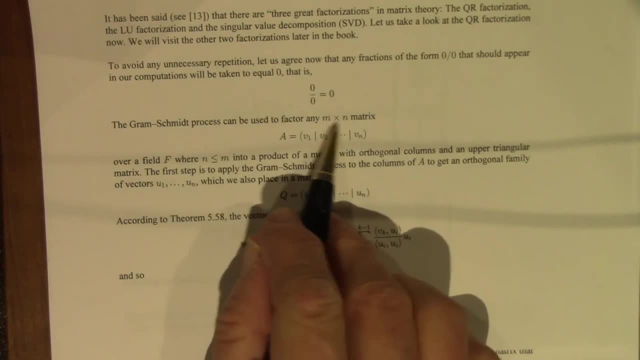 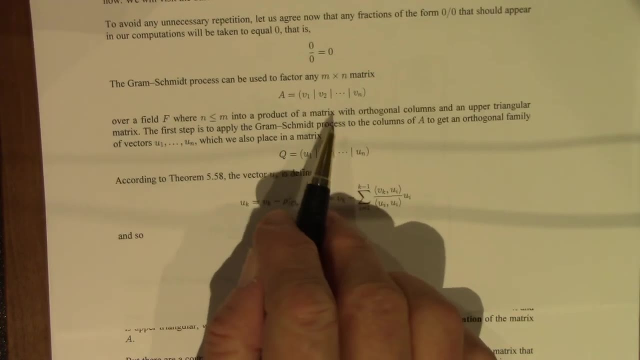 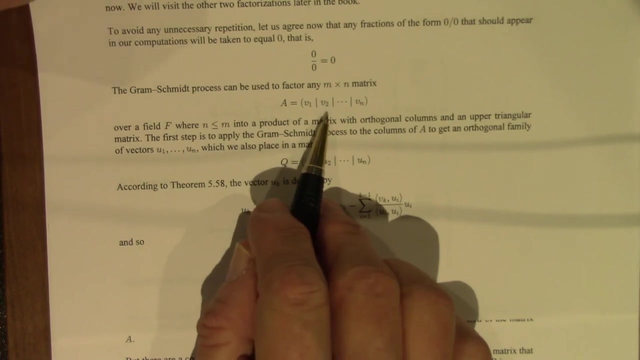 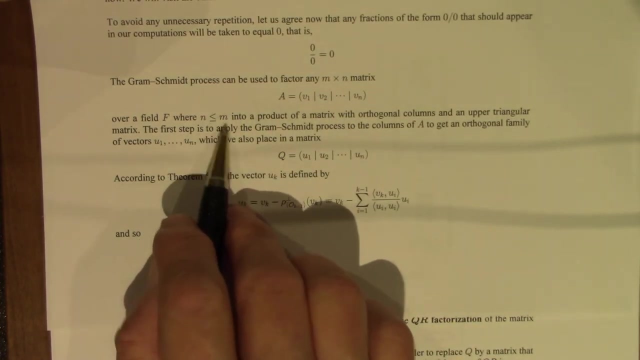 Okay, so suppose we have an m by n matrix and we'll write the columns this way. The Gram-Schmidt process can be used to factor this matrix as long as- and we're going to restrict our attention to n- less than or equal to m. 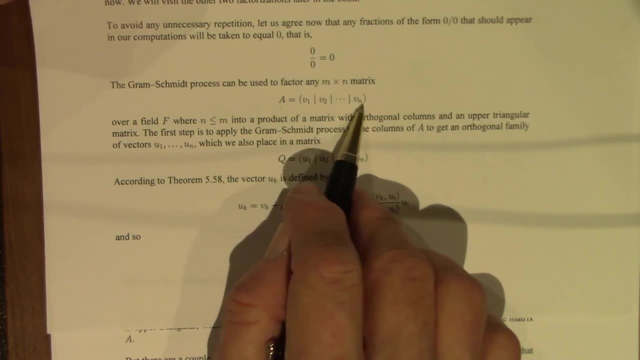 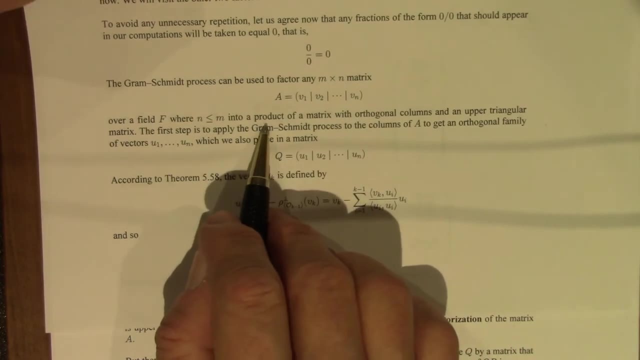 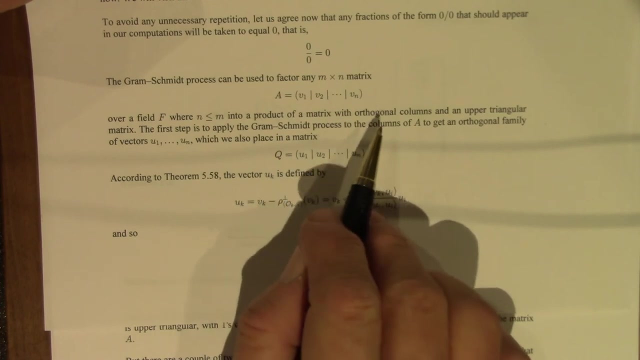 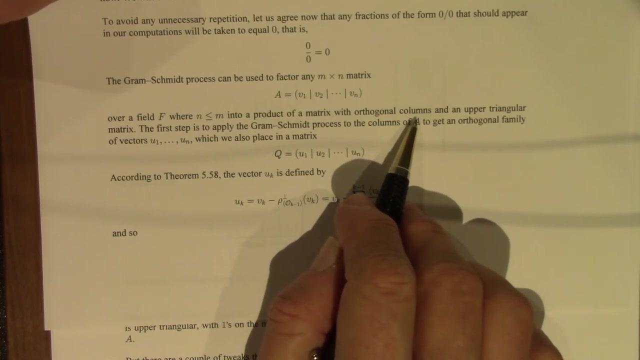 So the number of columns is less than or equal to the number of rows. We can use Gram-Schmidt to factor this matrix into a product, So we have a matrix with orthogonal columns. So some of the columns could be 0 columns. 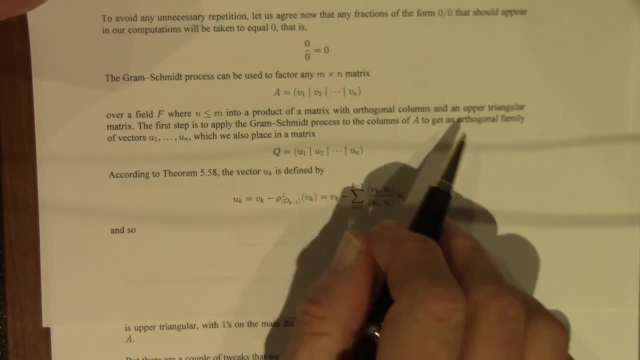 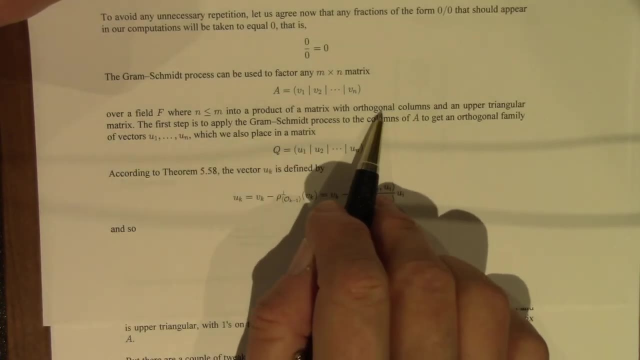 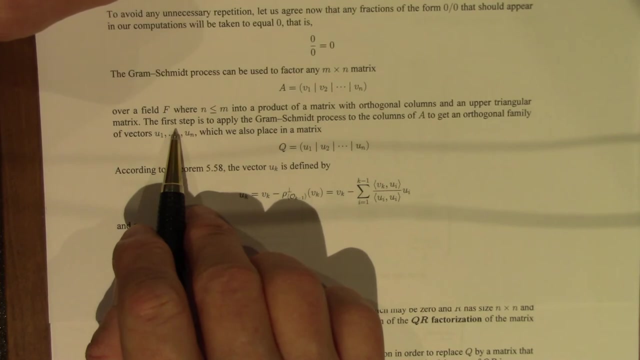 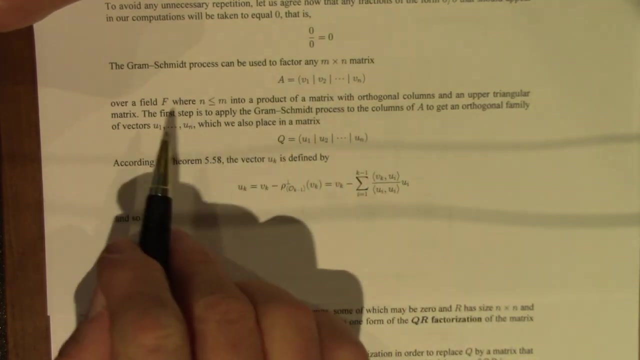 We'll address that issue- And an upper triangular matrix, So it'll be orthogonal times upper triangular. The first step in this process is to apply Gram-Schmidt to the columns of A And that will produce an orthogonal family of the same size. 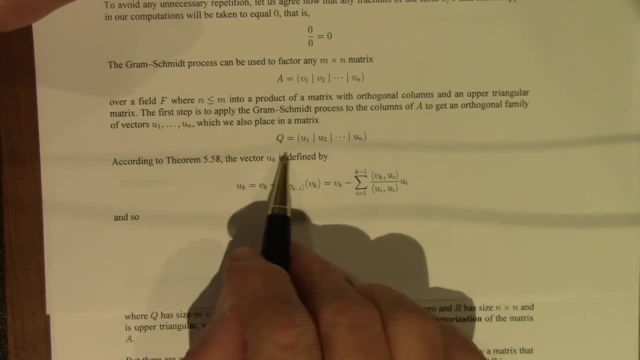 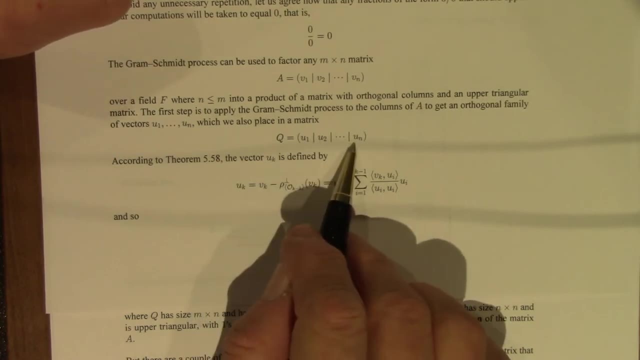 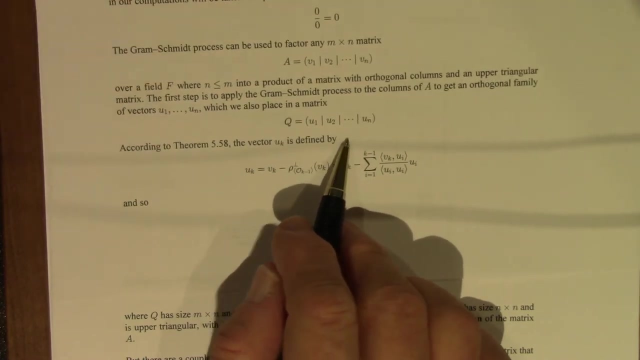 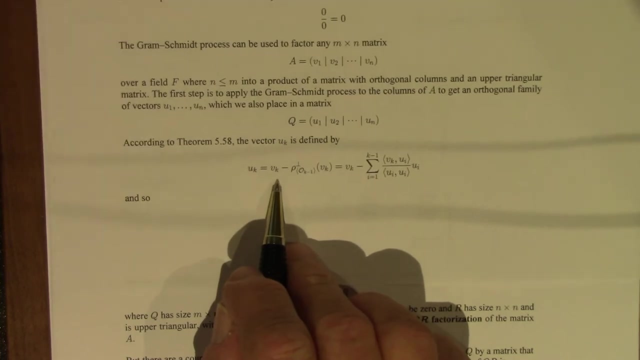 We don't cast out any 0 vectors And put that in a matrix which we'll call Q. So this has orthogonal columns. That is the left-hand factor in the decomposition. The actual columns here are given by this formula. It's the Gram-Schmidt formula. 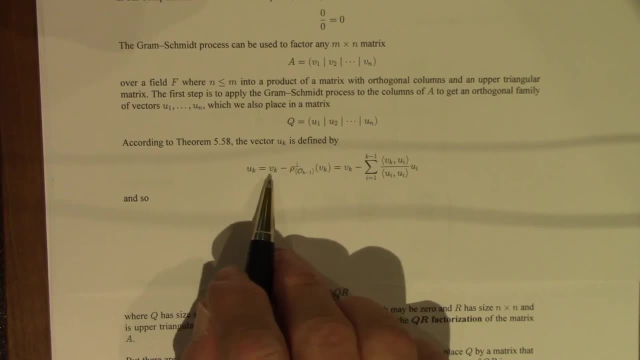 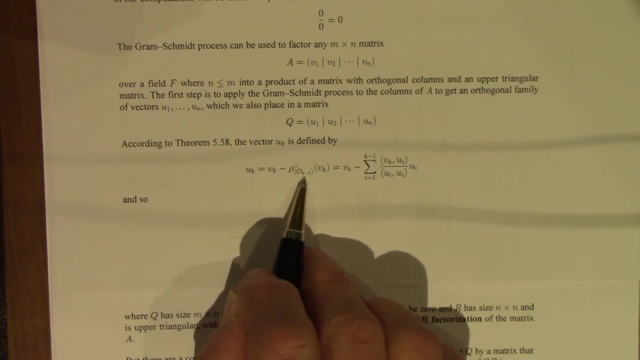 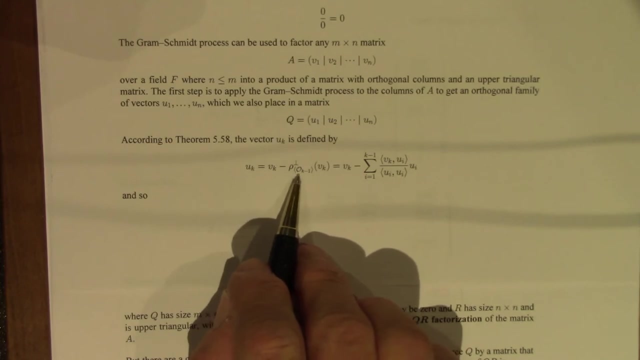 Uk is the residual vector vk minus the projection of vk onto this subspace, that is spanned by v1 through vk minus 1. Or equivalently. did I say that right, Spanned by v1 through vk minus 1. Or equivalently? 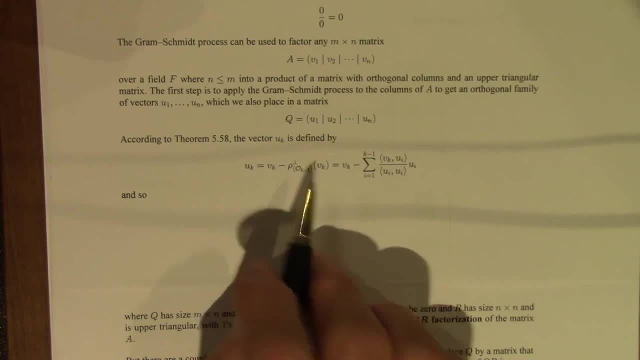 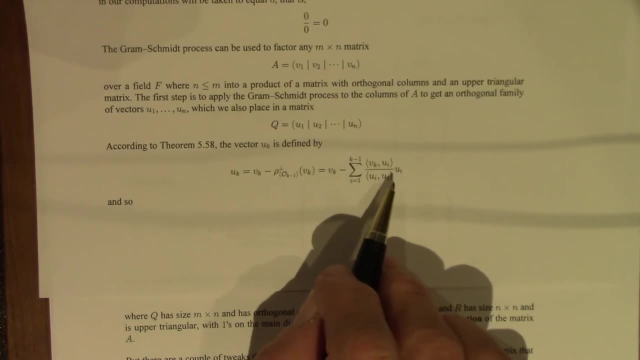 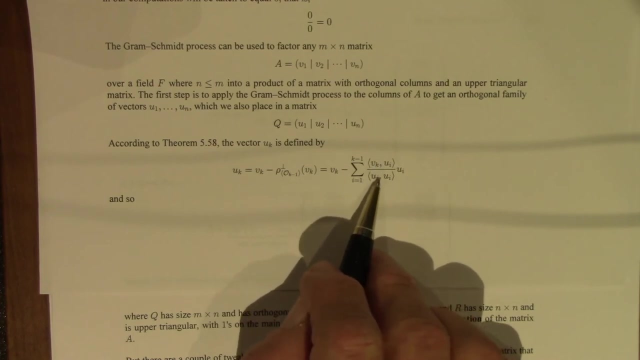 u1 through uk minus 1.. And this is the formula. If ui is 0, then this term is 0. You'll have a 0 over 0 here, And so we can't get upset about that and say it's undefined. 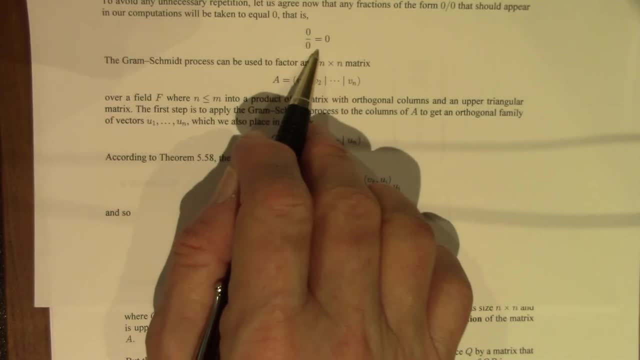 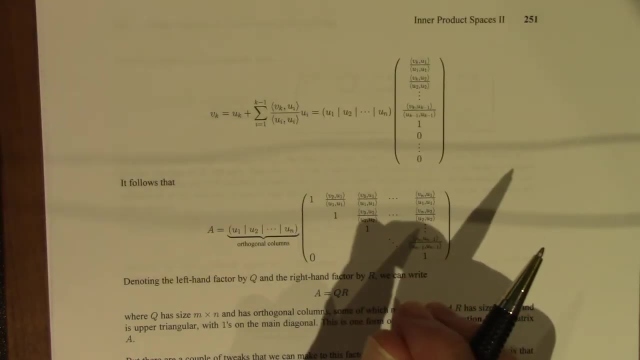 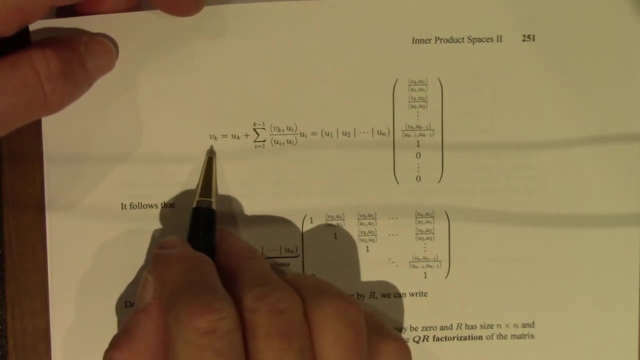 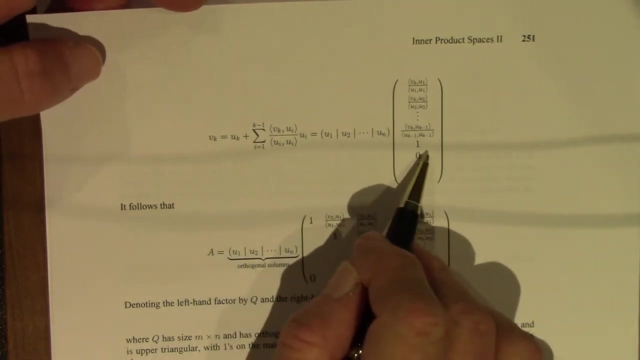 That's why I introduced this little temporary convention. Now, if I solve that equation for vk, vk is uk plus this same sum, And this I can write as a product of two matrices: The matrix here whose columns are the orthogonal vectors u1 through un. 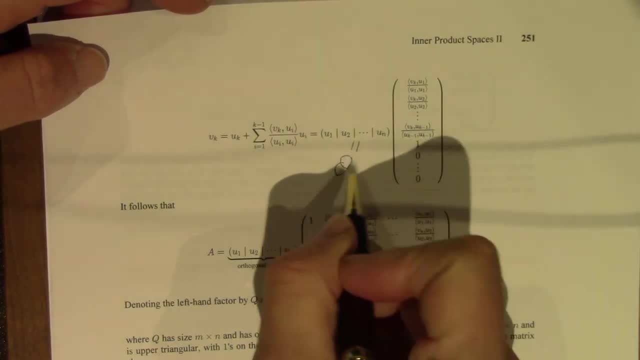 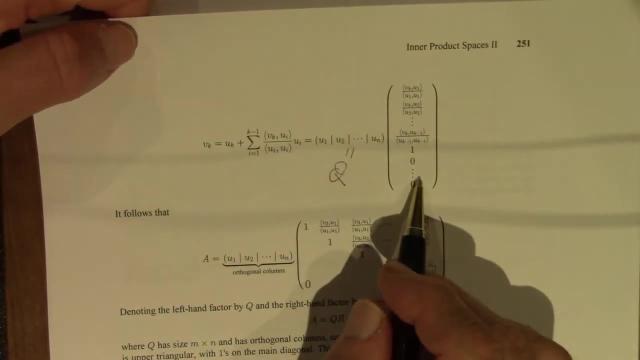 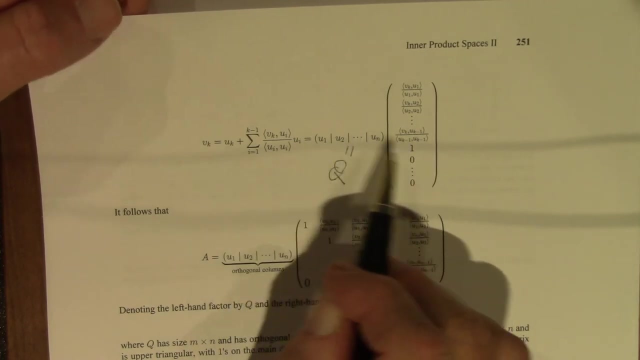 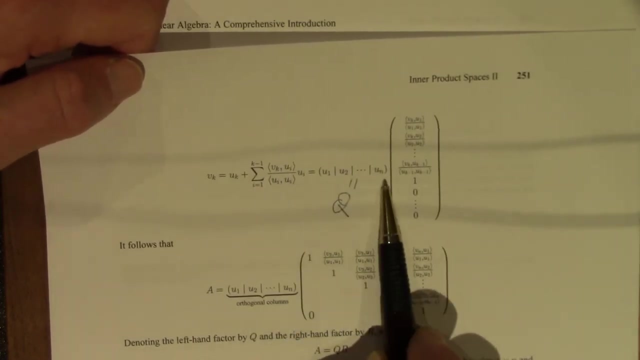 this is q times this matrix And if you take this product, this is a single column. So to take this product and there's various ways, but what I would suggest you do when you think about why this is equal to this product. 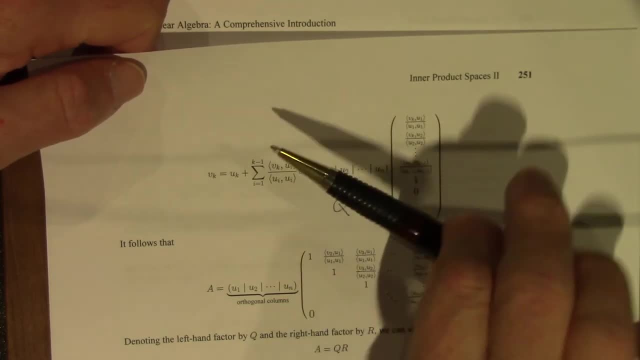 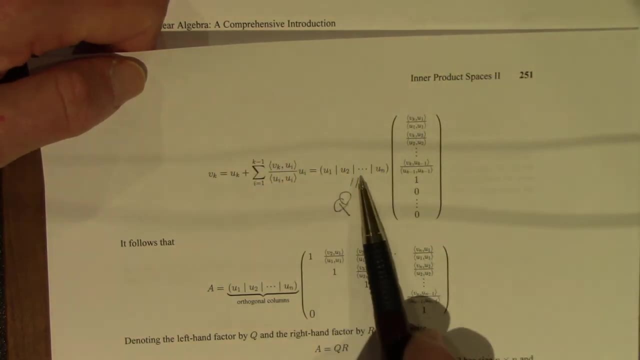 is to take this column and rotate it 90 degrees and lay it on top of here and march down the rows of q And you will see that this is what you will get. Okay, For the kth column, for vk, vk. 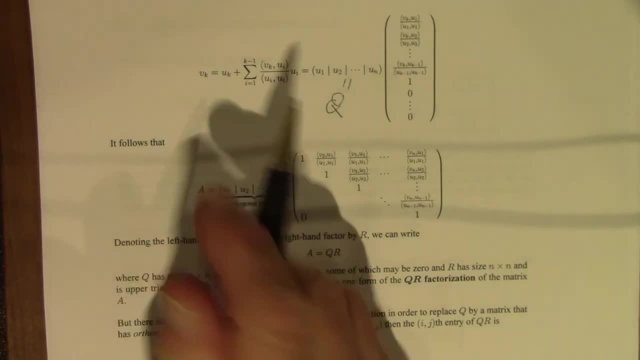 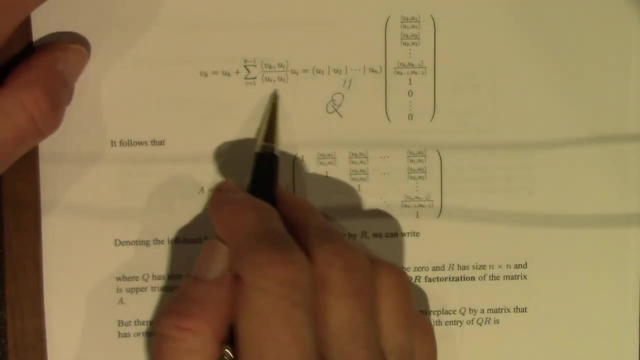 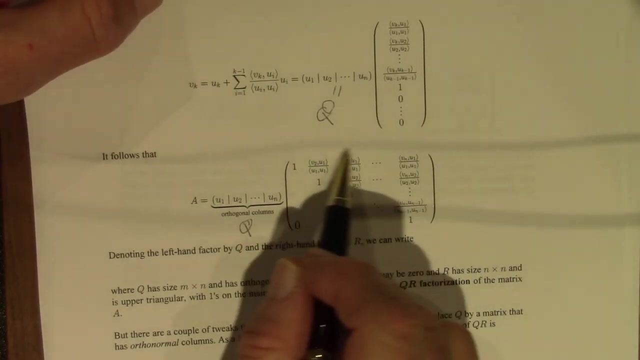 Well then, the entire matrix A, which is- let me go back here- A is, its columns are v1 through vn, then we get q again here times this matrix, which just is: this is the kth column, so the first column. 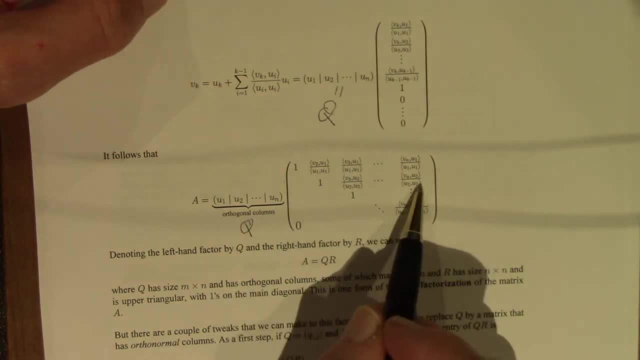 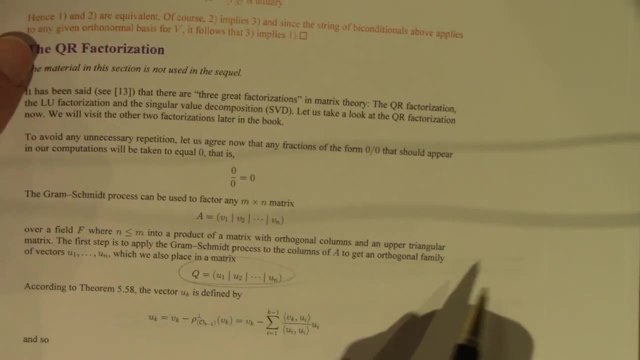 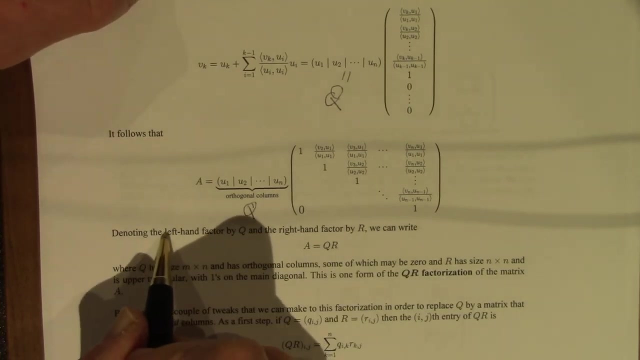 second column, third column and so on. This is what these look like. Okay, I guess I've already said that this is q, So I don't need to say denoting the left-hand factor by q, So we'll just denote. 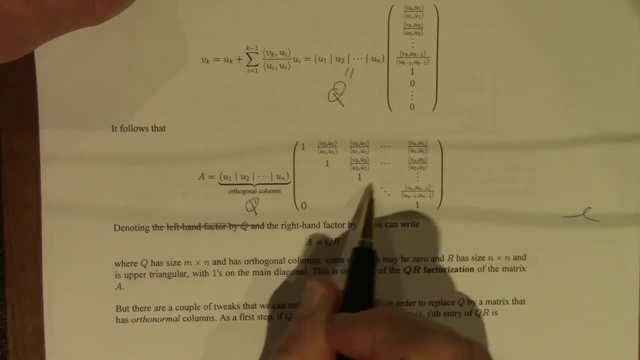 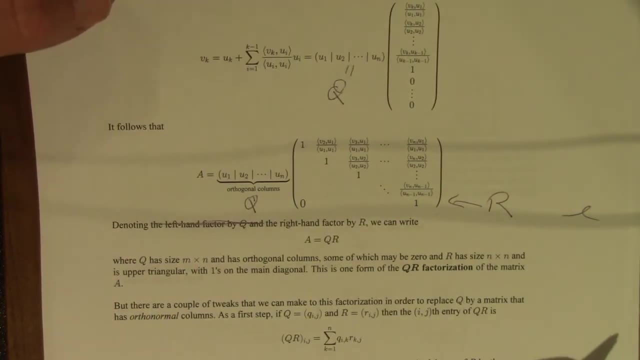 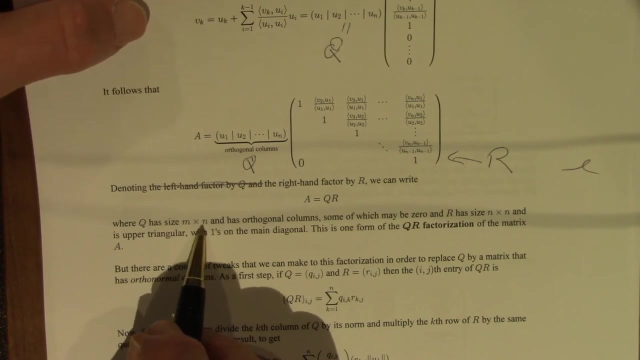 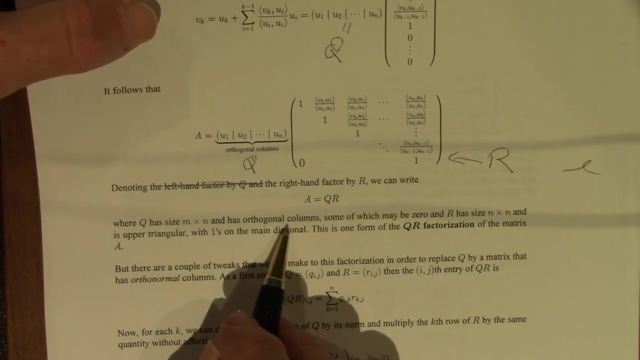 the right-hand factor by r, So we're going to call this matrix r. So we have qr, It's the qr factorization. Okay. q has size m by n, the same as A, and it has orthogonal columns, some of which may be zero. 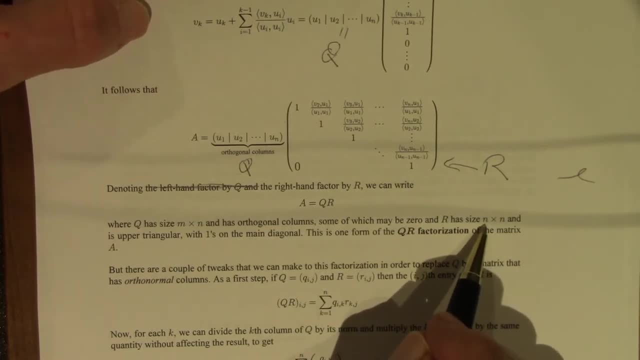 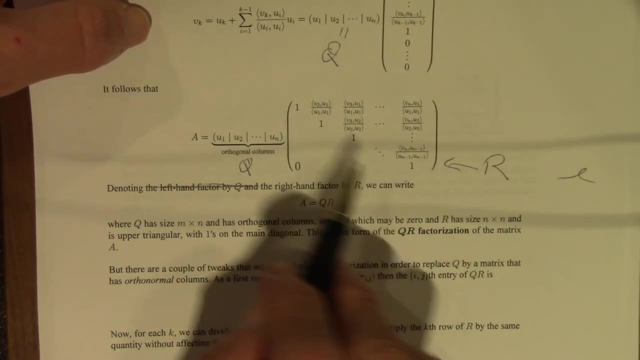 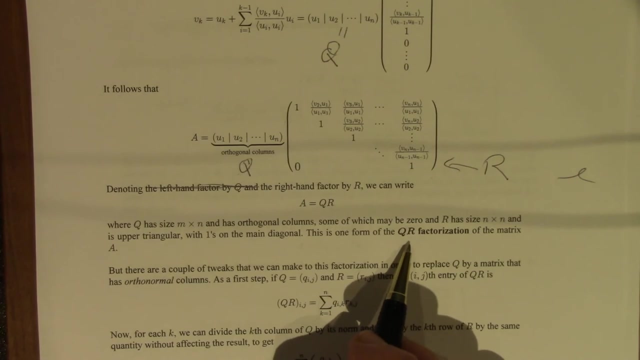 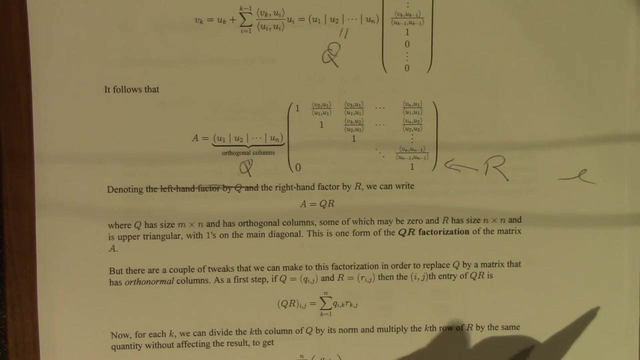 And r is a square matrix size n by n, and it's clearly upper triangular with ones on the main diagonal. So this is one form of the qr factorization. Now there's one thing that's a bit disturbing about this, and that is the fact that 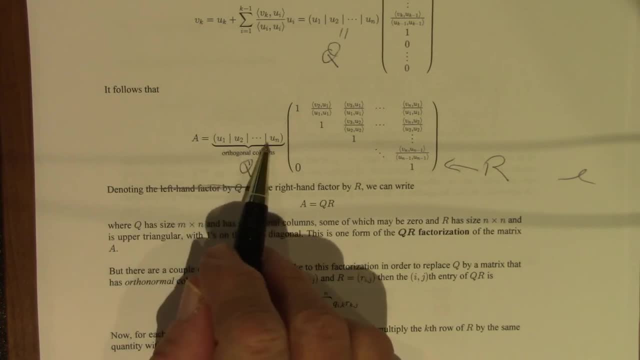 some of these columns might be zero. I suppose it's also modestly disturbing that these don't have to be orthonormal columns, the non-zero ones. Well, it's easy enough to normalize, So we're going to normalize the non-zero columns. 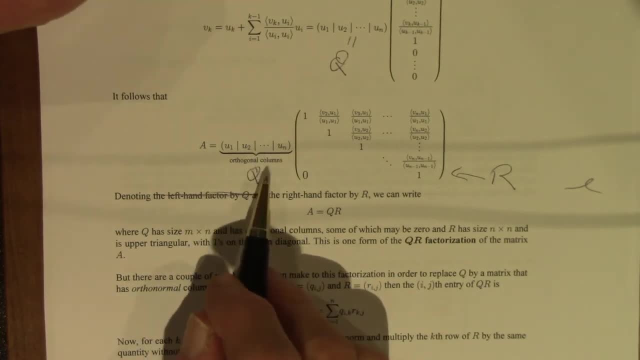 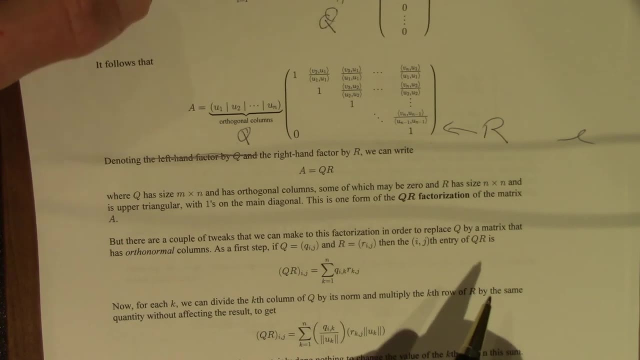 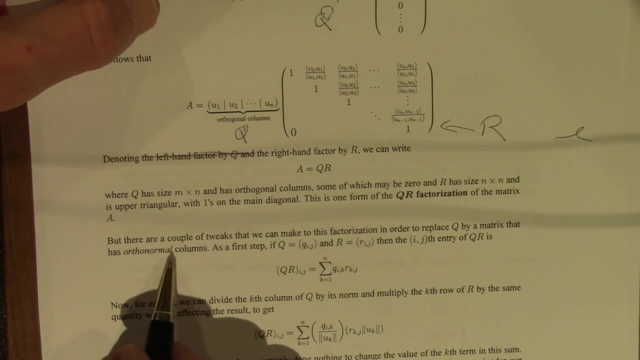 and then we're going to deal with the zero columns. So that's why I say there's a couple of tweaks that we can make to this factorization in order to replace q by a matrix that has orthonormal columns, So all the columns. 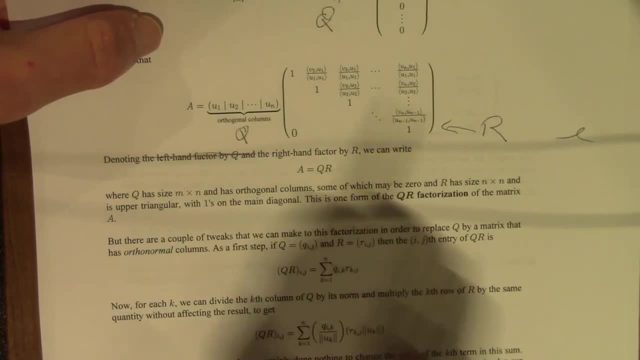 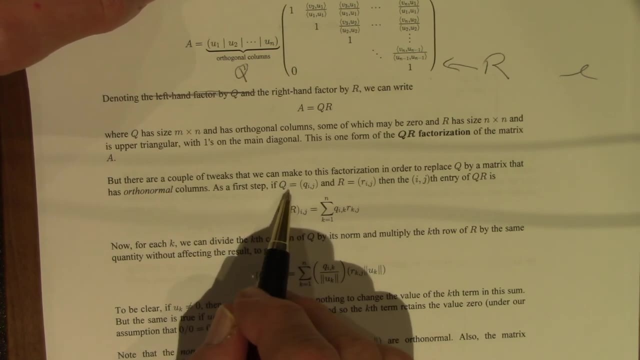 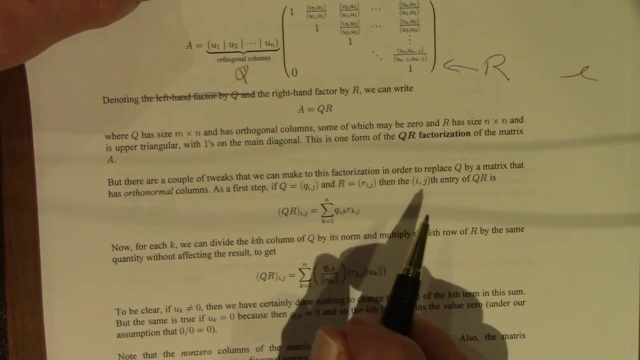 form an orthonormal set, which means none of the columns are zero. So the first step is, if I denote the entries of q by little qij and the entries of r by little rij, then the ijth entry of this product, qr. 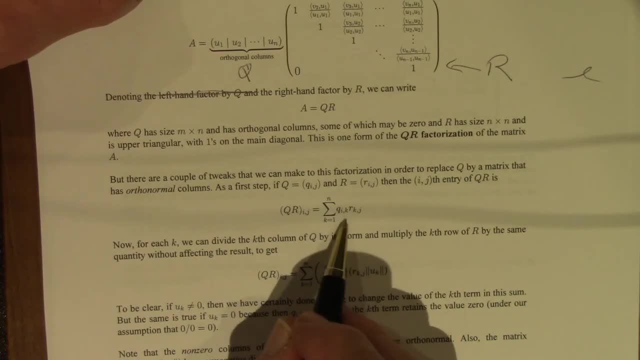 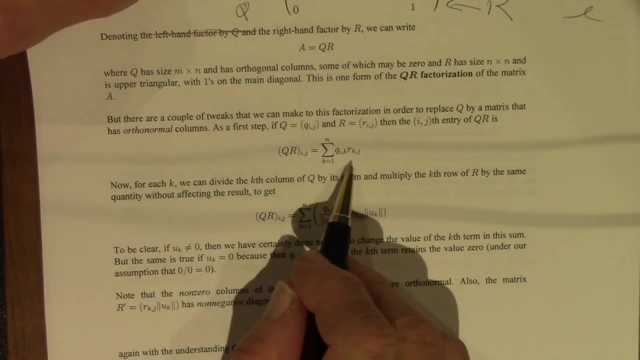 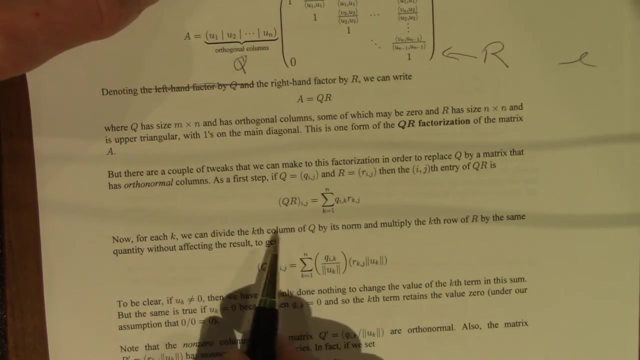 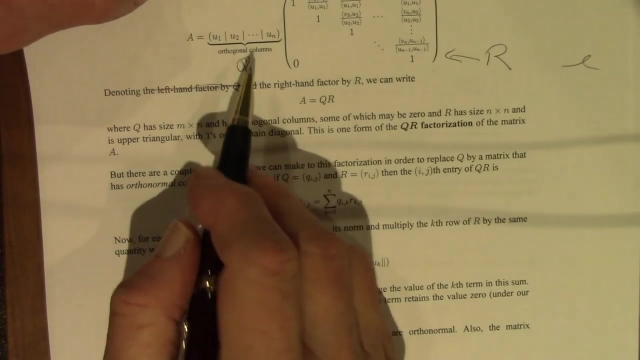 or indeed a looks like this: This is just the ordinary formula for matrix multiplication. Now for each k in this list here of columns, we can divide the kth column of q by its norm. When a column is zero, we're dividing by zero. 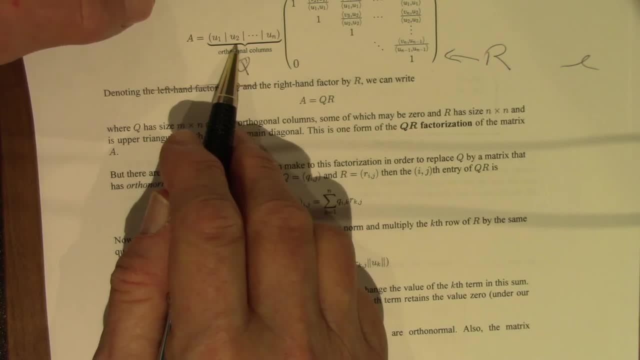 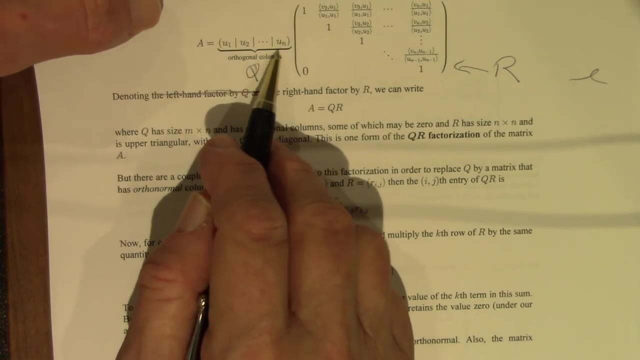 So we have zero over zero, which we are thinking of as zero. So normalizing all of the columns by our convention simply normalizes the non-zero columns in the usual way and doesn't do anything to the zero columns. That's why I wanted. 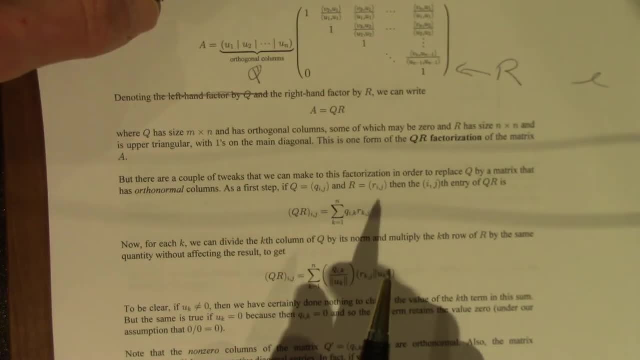 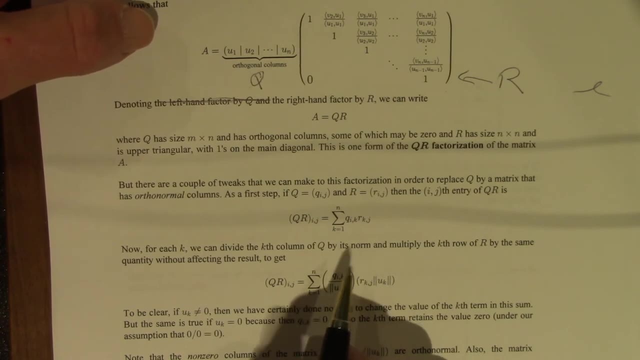 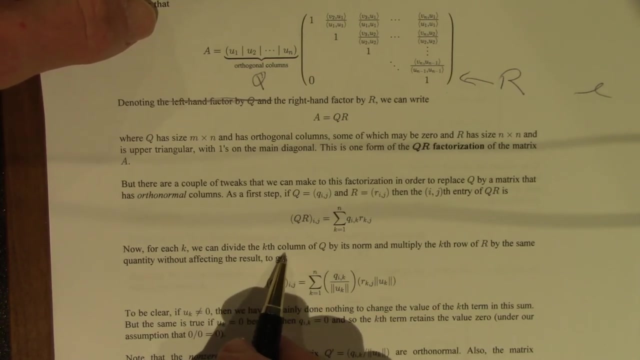 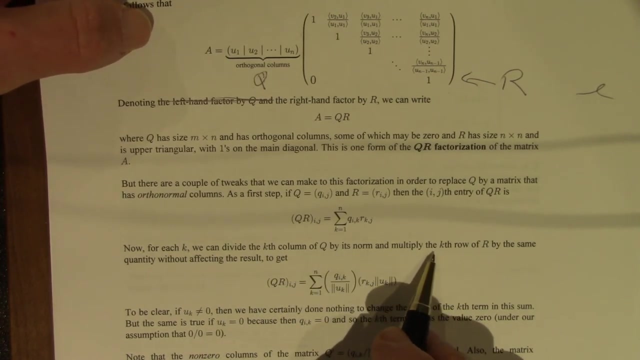 zero over zero to be zero. So I could have said what I just said instead, but it's simpler if I introduce that convention. Well, if we're going to divide a kth column of q by its norm, then we need to multiply. 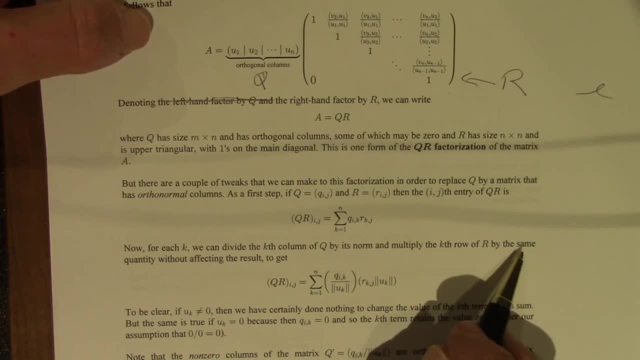 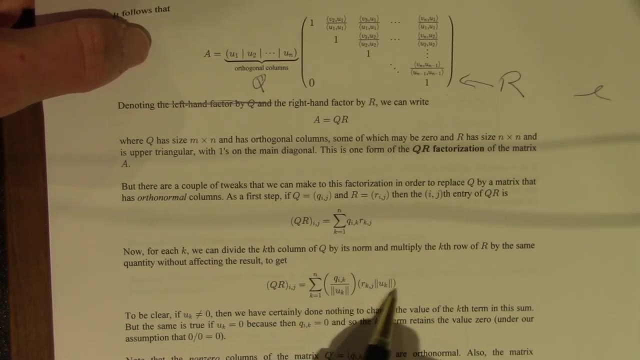 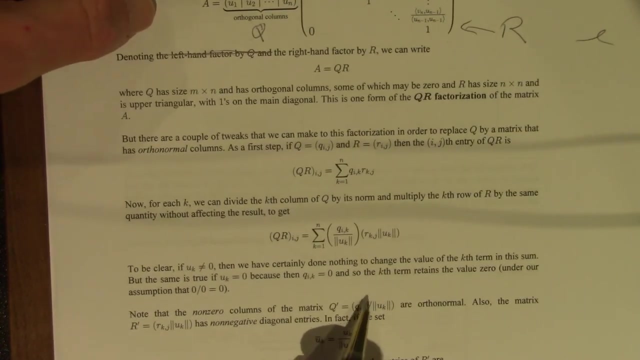 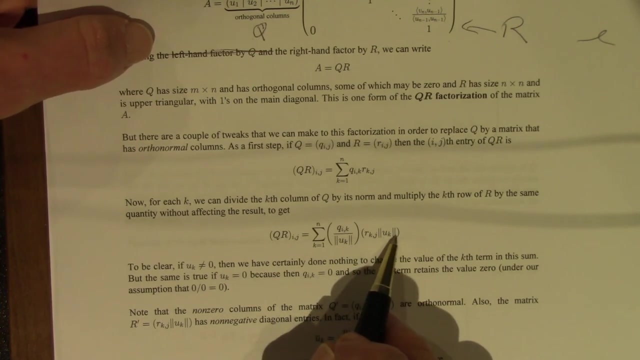 the kth row of r by that same norm. So the ijth entry of qr will simply look like this, and we have done nothing To be clear about that: if uk is non-zero, then clearly we're just dividing and multiplying by a positive number. 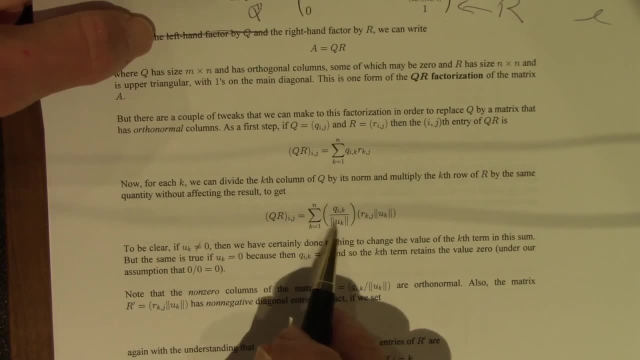 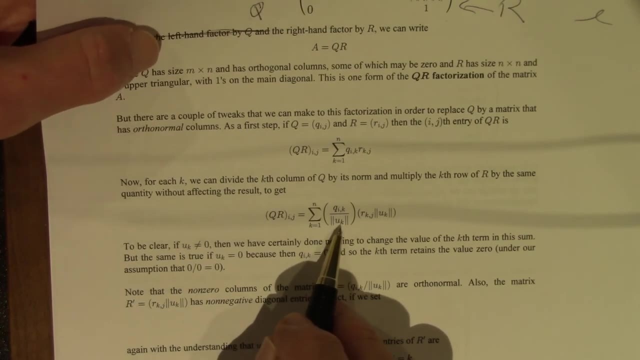 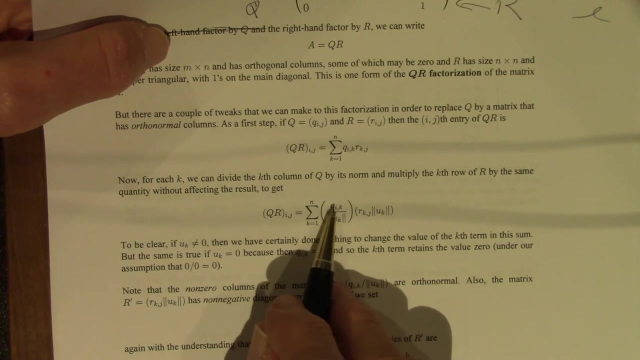 So that does nothing. But when uk is zero, qik would be zero because it's one of the entries in the column uk. So this was zero anyway. it was zero up here and now it's zero over zero times zero. so it's still zero. 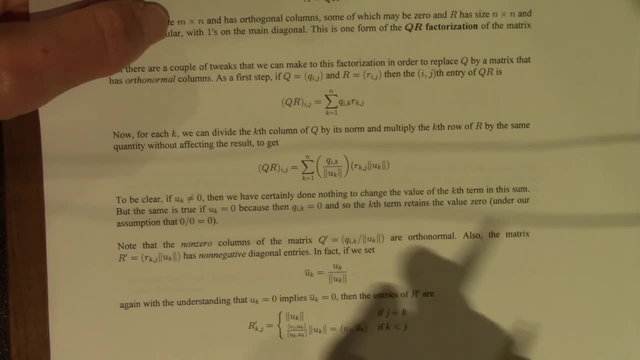 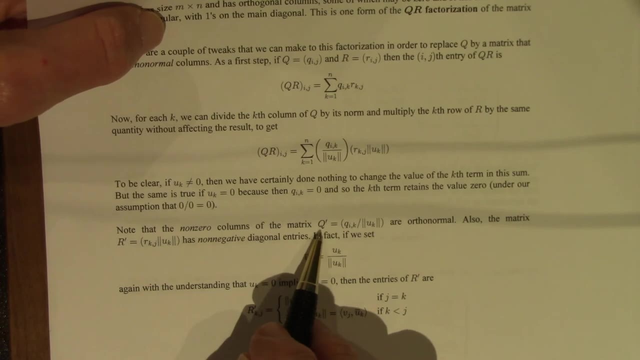 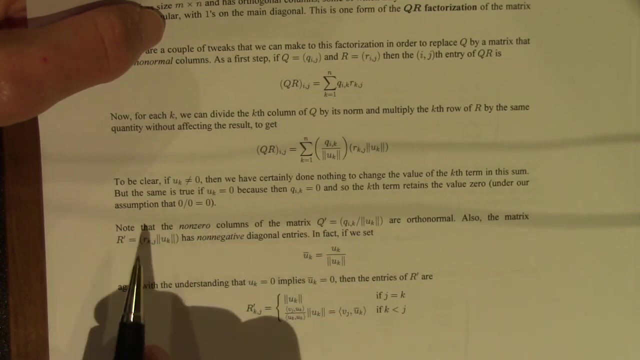 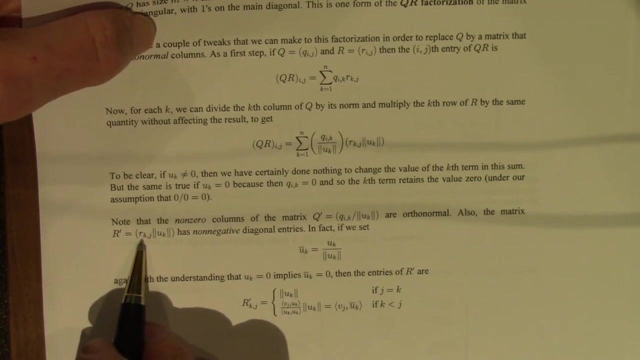 So we haven't changed that either. The non-zero columns of the new matrix, which I call q' looks like this: they are orthonormal. And the new matrix, the new r matrix, r' where you multiply r, k, j. 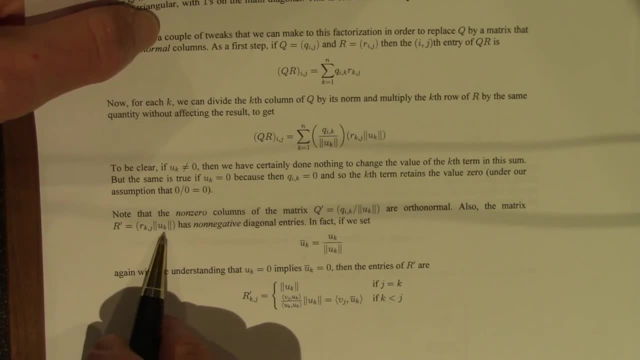 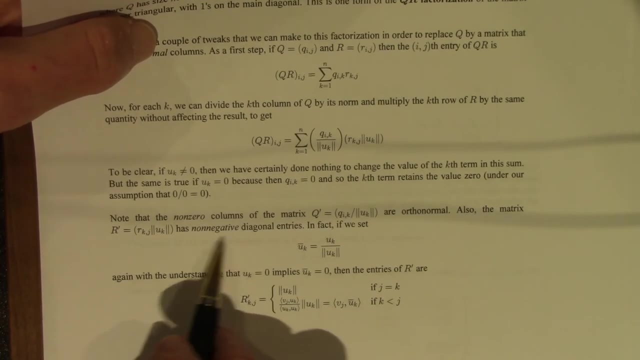 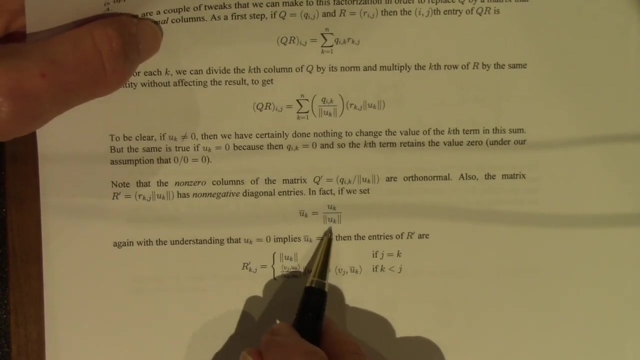 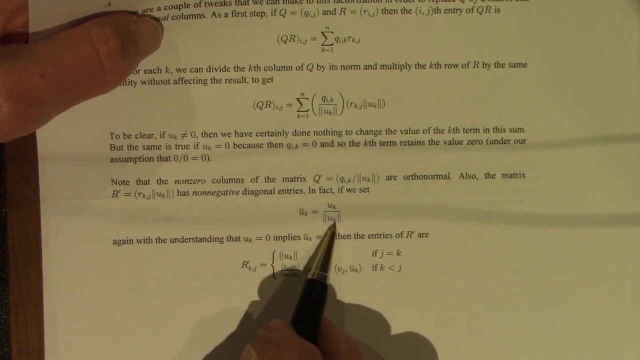 by the norm of uk. some of those norms may be zero. so the best we can say is that r' has non-negative diagonal entries And if we set, just for convenience, uk bar to be uk over norm of uk and again, 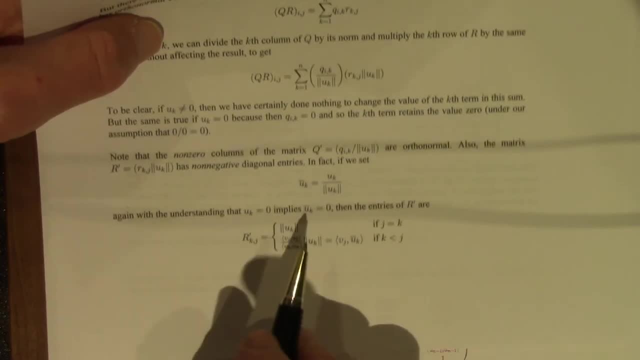 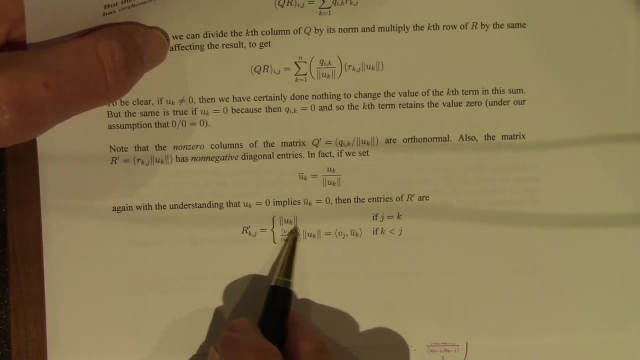 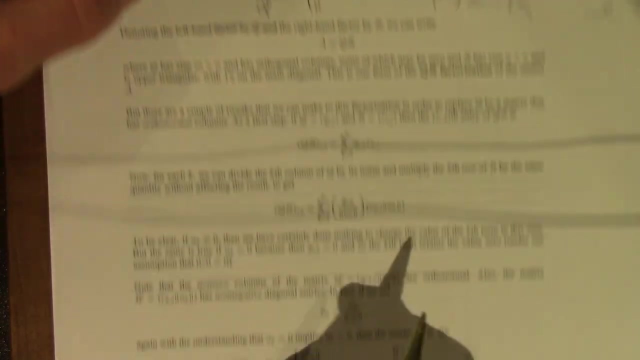 if uk is zero, uk bar is zero, then the entries of r' look like this On the diagonal: they're the norm of uk because we have multiplied these ones by the appropriate norms And the other locations we're multiplying by uk. 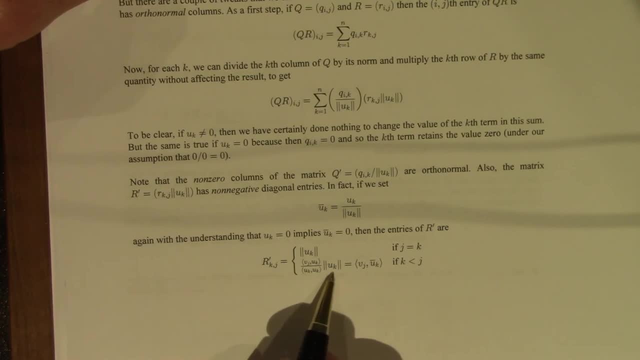 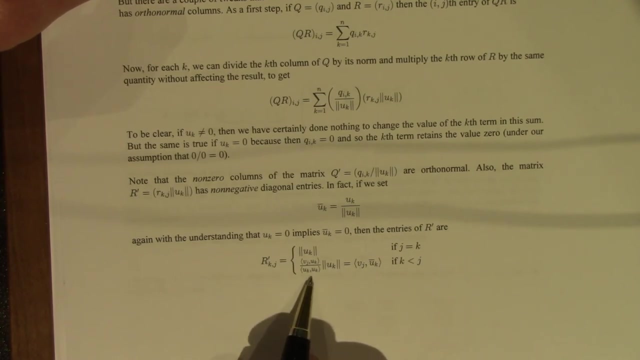 I'm sorry, the norm of uk. so it looks like this, which can be simplified notationally a little bit by this: This denominator is the norm of uk squared, so there's a cancellation and then we pull in the norm of uk. 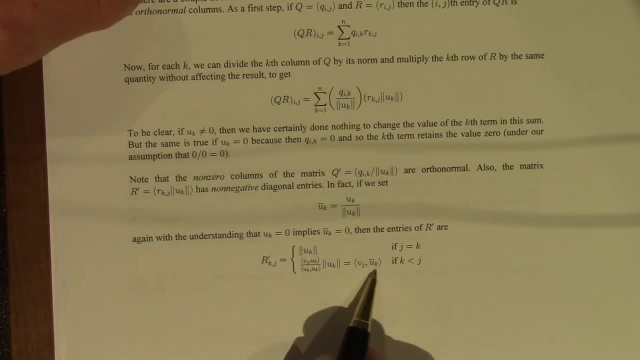 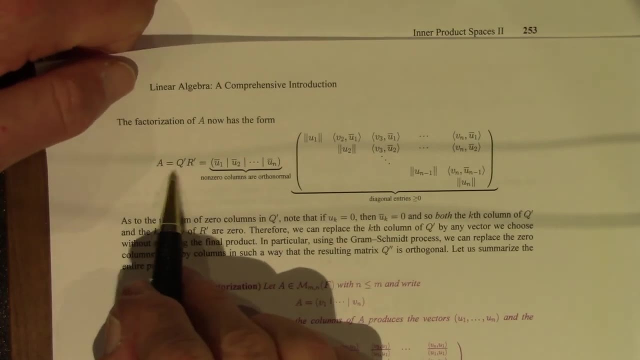 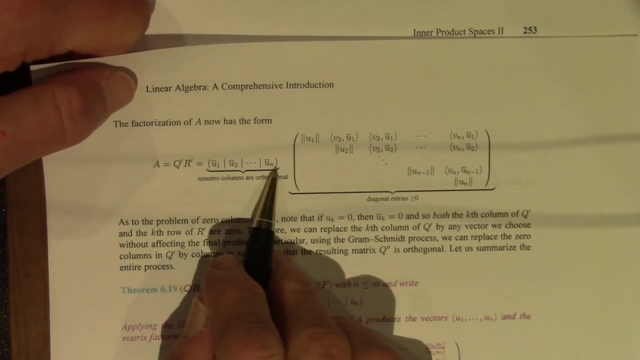 in the second coordinate. here It looks like this: So this new factorization: a equals q, prime, r, prime. now we have the uk bars here. They have the property that the non-zero columns are orthonormal, because we've normalized the non-zero columns. 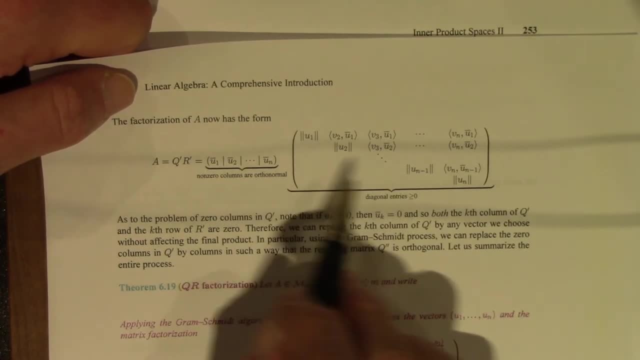 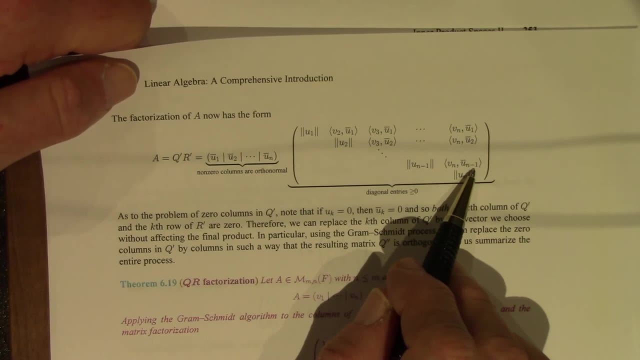 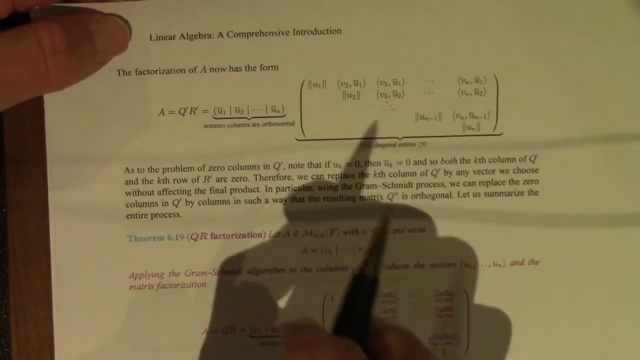 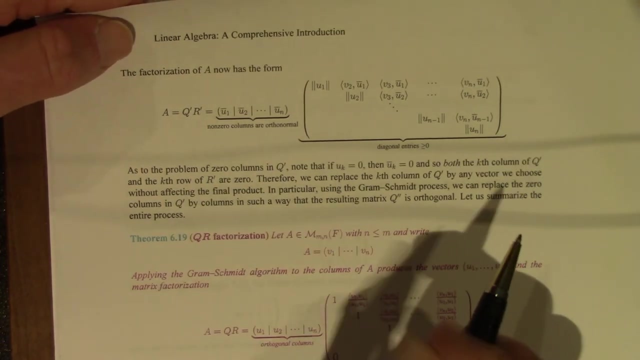 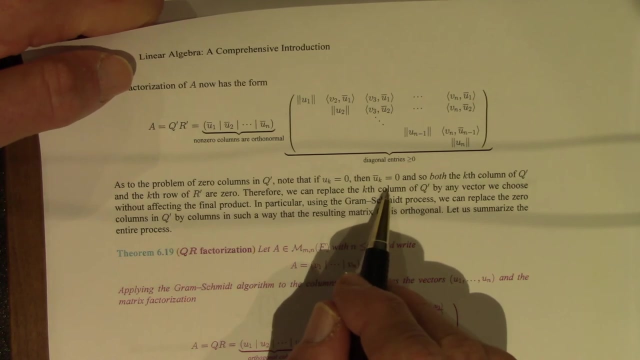 and this is the resulting r prime matrix and you can see the norms on the diagonal and the rest here. As to the problem of zero columns in q prime, if uk is zero then uk bar is zero and conversely, So these are zero at the same time. 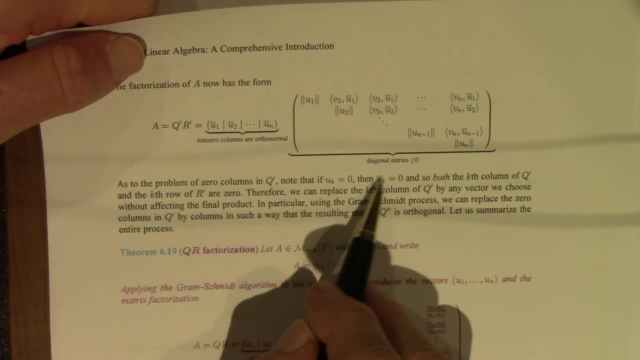 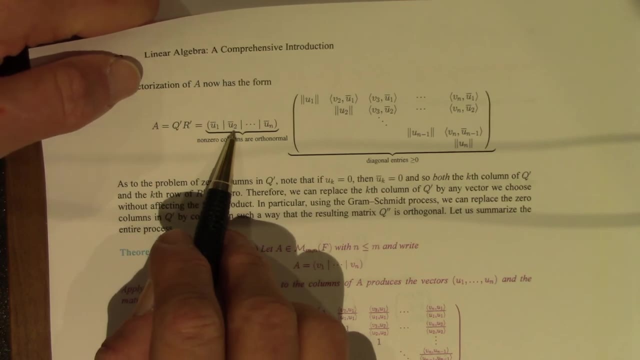 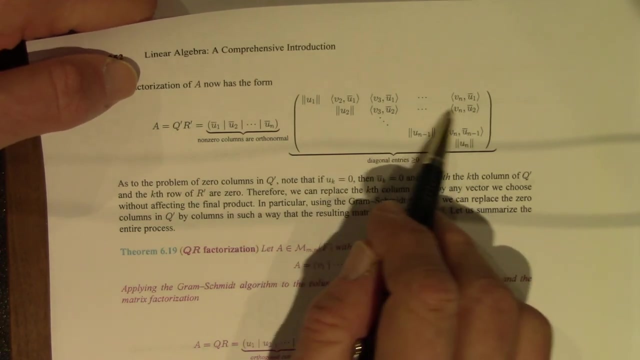 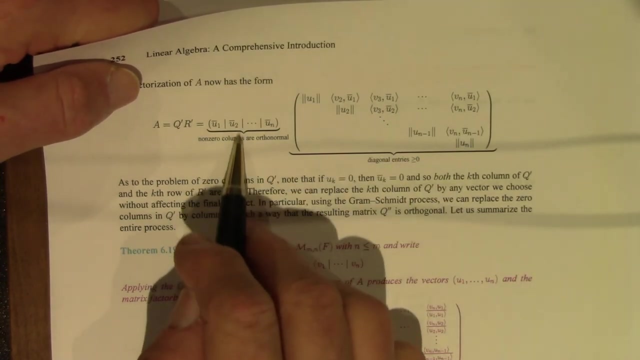 So, in particular, if uk is zero, uk bar is zero, then we've got those uk bars in the second coordinates. here We've got norm of uk. here The whole row is zero. If the kth column is zero, the kth row is zero. 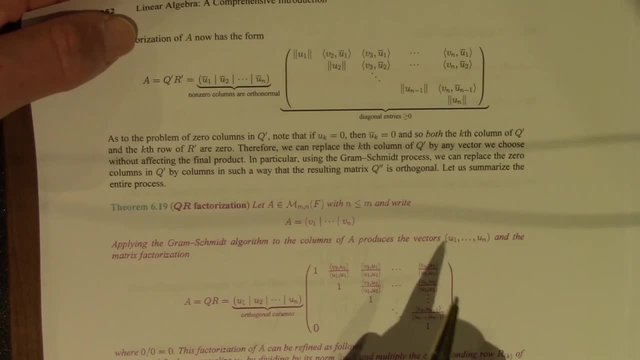 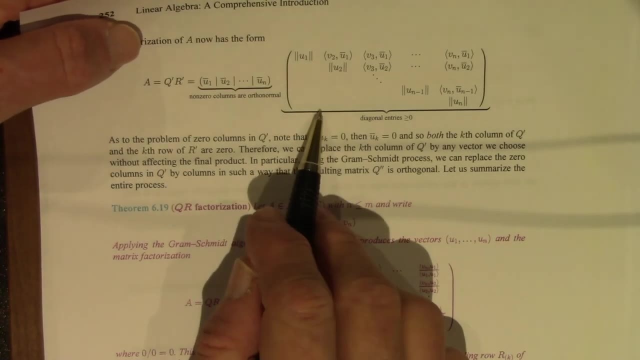 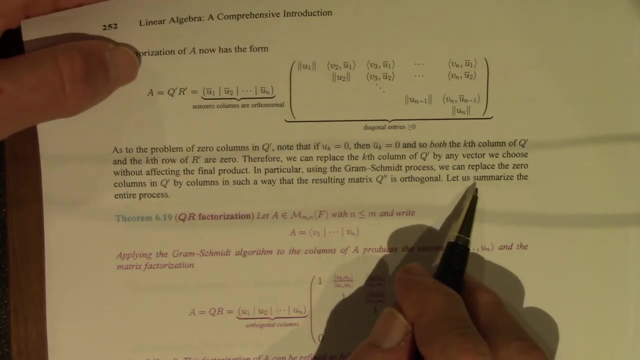 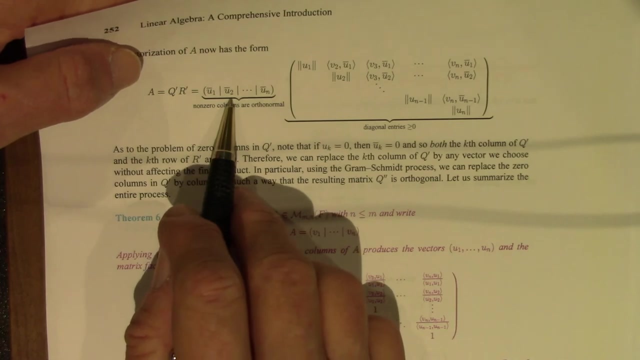 Well then, if you think about how matrix multiplication works, you can see that matrix multiplication works, and I'll leave this for you. The interaction of the rows and the columns in the product tells us that we can replace a zero column by anything we want. 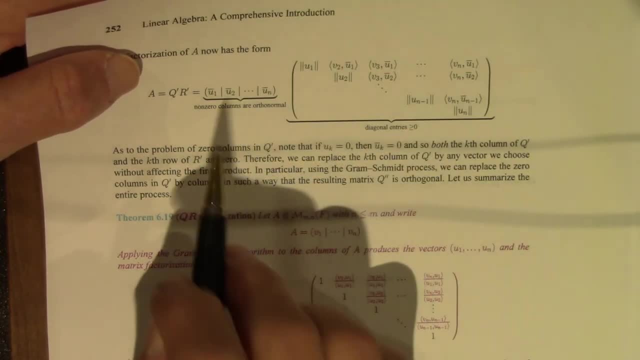 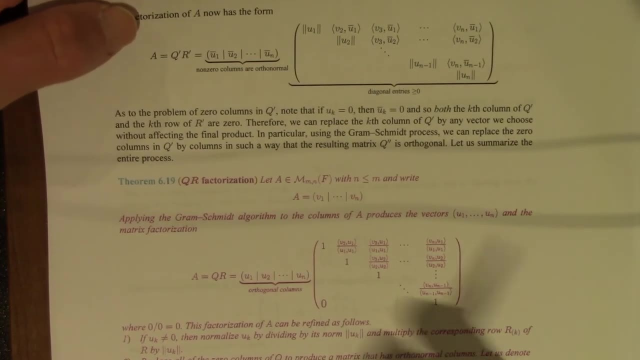 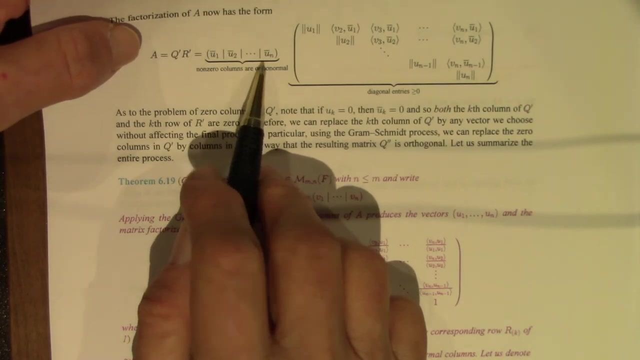 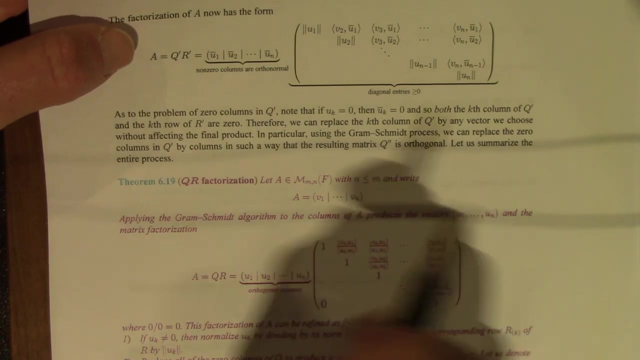 As long as that we don't touch the zero row, the matrix product will be the same. So what we can do is take the non-zero columns, which are orthonormal, and extend that those to an orthonormal basis, or I'm sorry? 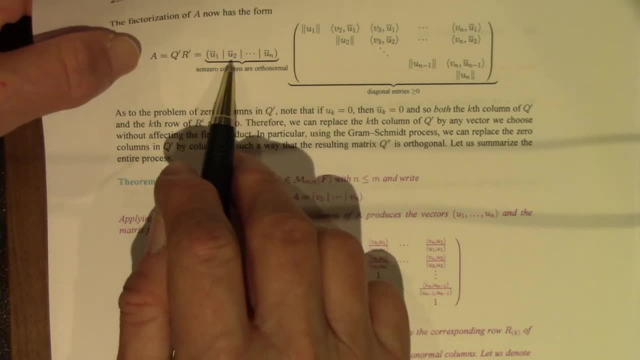 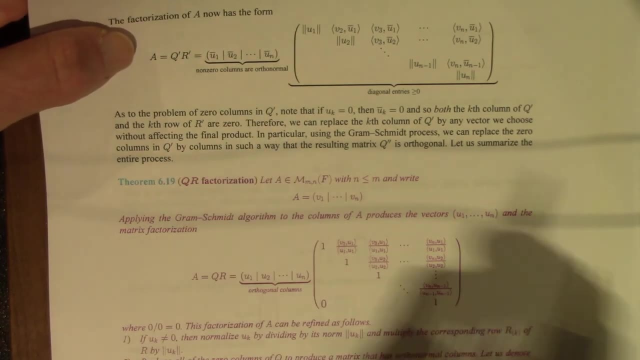 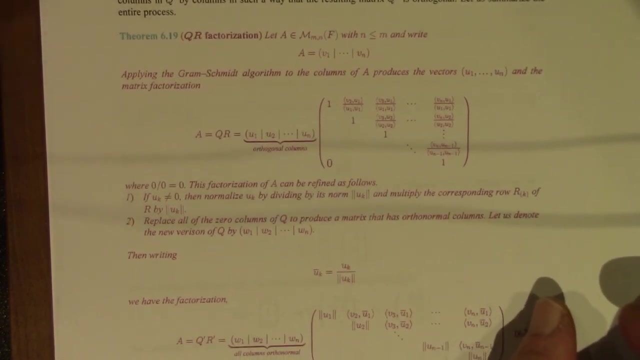 extend it to an orthonormal set by replacing the zero columns by the appropriate vectors which we can get from the Gram-Schmidt process, for example. So here is the summary, and this is a little testy. I rewrote this several times. 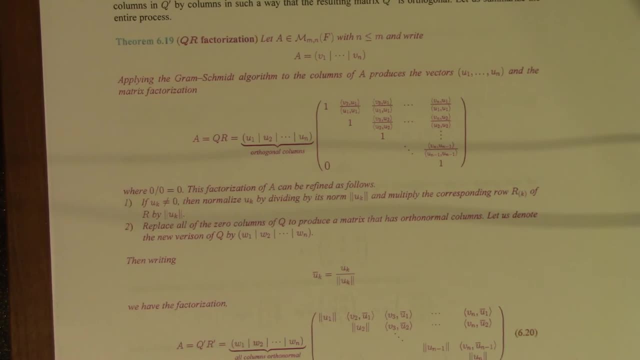 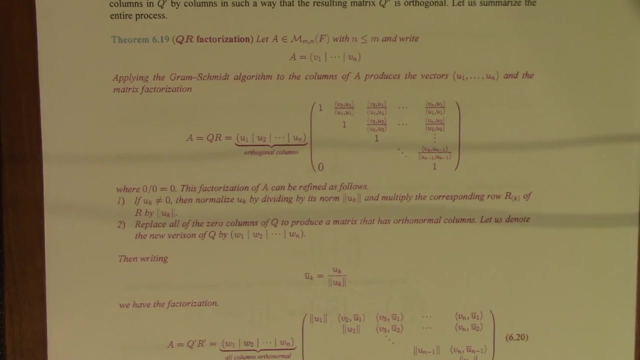 to try to make it as clear as I could. It's something you're probably going to need to go over more than once if you are interested. Again, this is material. This is extremely important. It was not referred to as one of the three great factorizations. 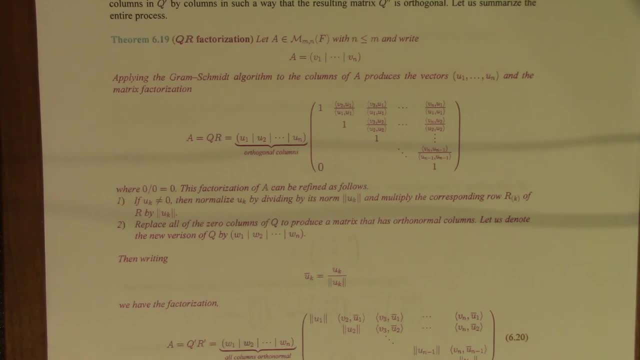 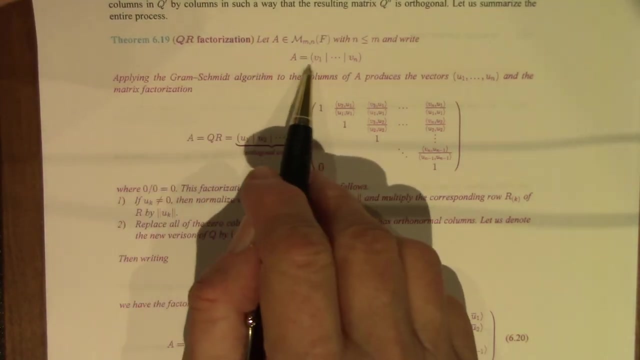 in matrix theory for nothing, but we're not going to be concerned with it in this course, which is more theoretical than it is applied. Here is a summary of the QR factorization. We start with a matrix in column form. There are fewer. 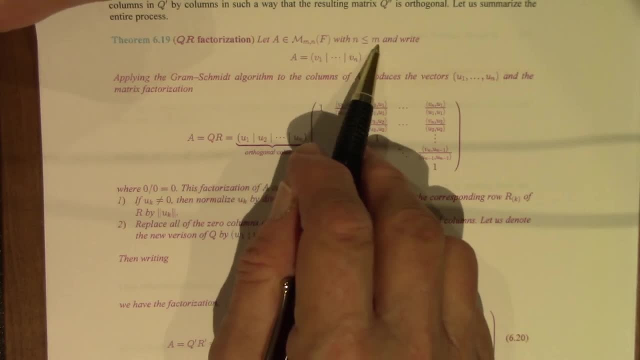 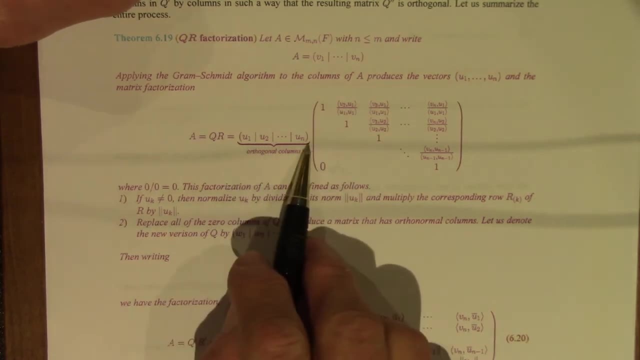 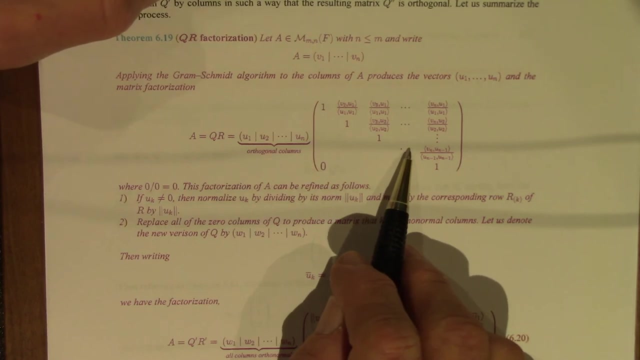 The number of columns is less than or equal to the number of rows. We apply the Gram-Schmidt algorithm producing orthogonal vectors. We place in this matrix Q. Here is R. This is just another way to write the Gram-Schmidt process. 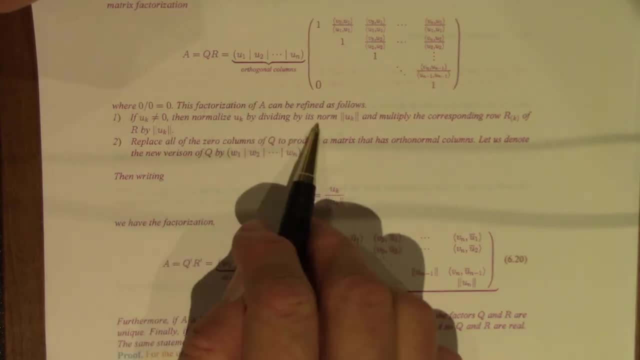 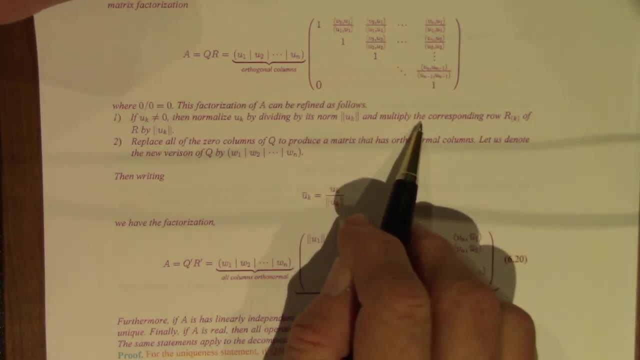 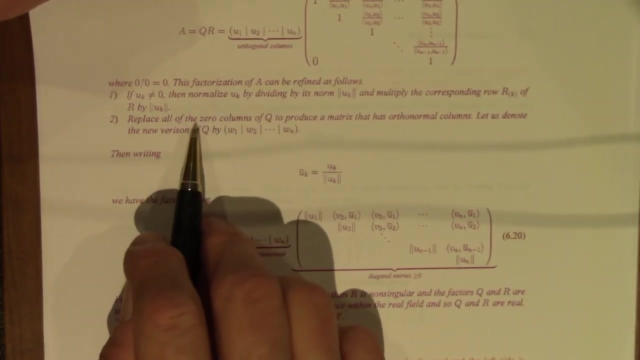 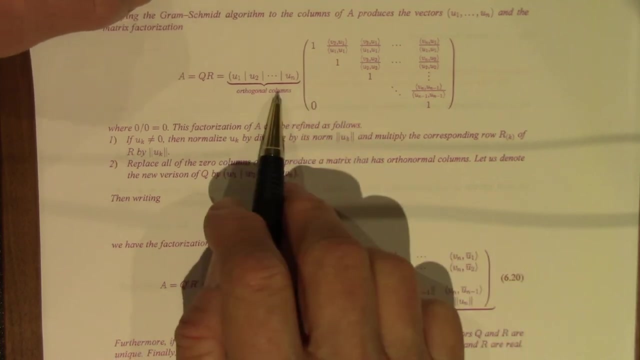 If a column is non-zero, we normalize it, and then we multiply the corresponding row of R by that same value. Second, we: This is a perfectly good QR factorization, but it's not quite what we want, So we do the number one here. 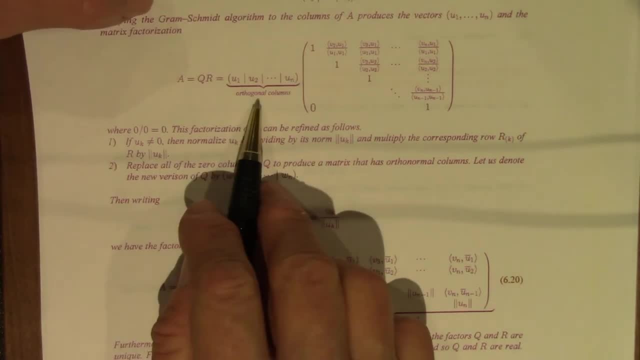 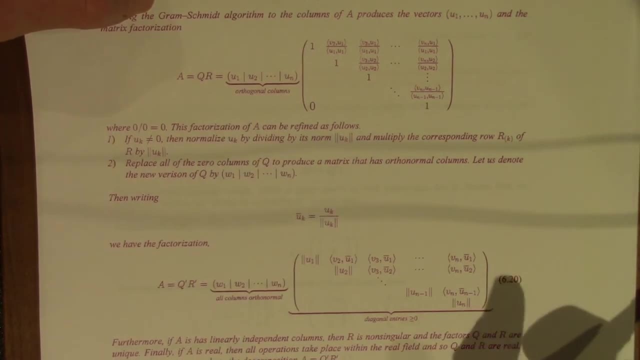 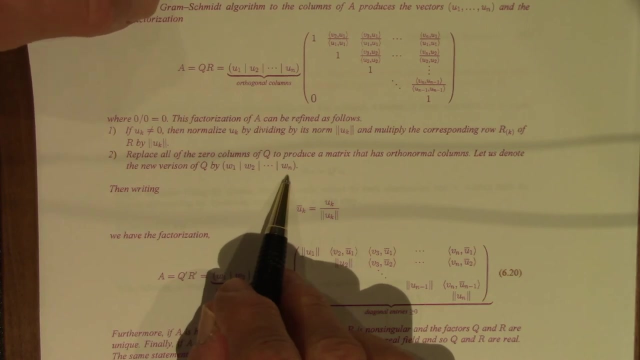 and then number two. we also replace all the zero columns of Q to produce a matrix that has orthonormal columns, And I'll denote that by W1 through Wn. Then again, with this notational convention, we produce this factorization. 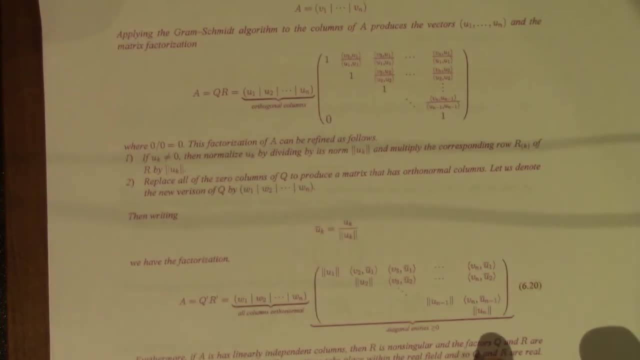 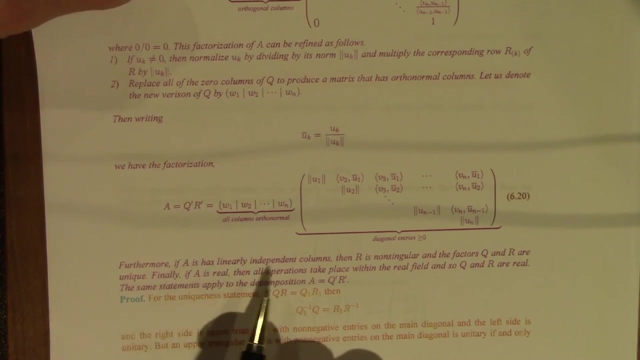 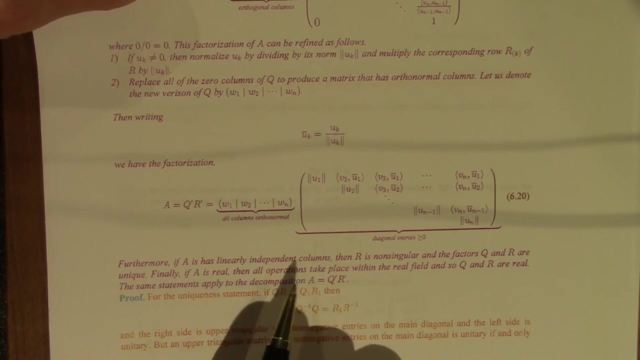 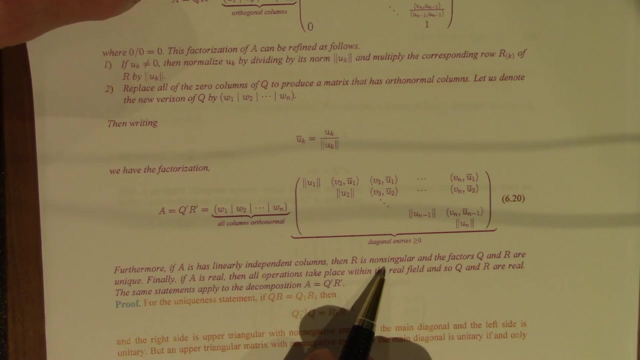 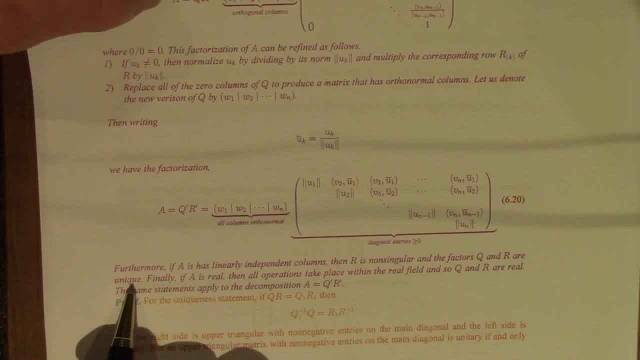 It's the same one as up here. I just copied it. Now, if A has linearly independent columns, if the original matrix has linearly independent columns, then R will be non-singular and the factors Q and R will be unique. 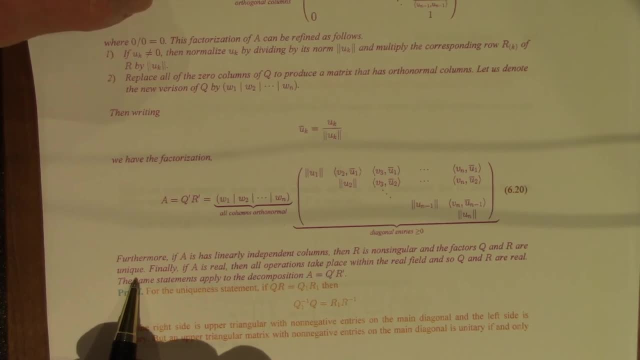 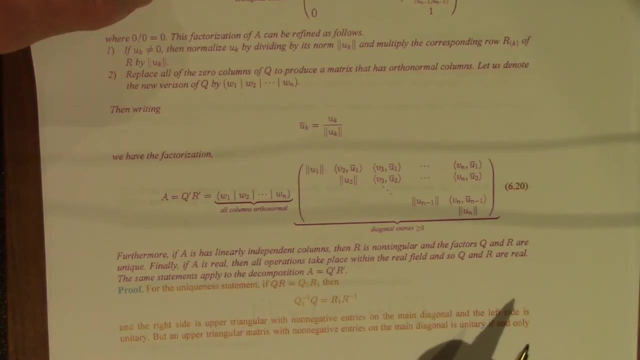 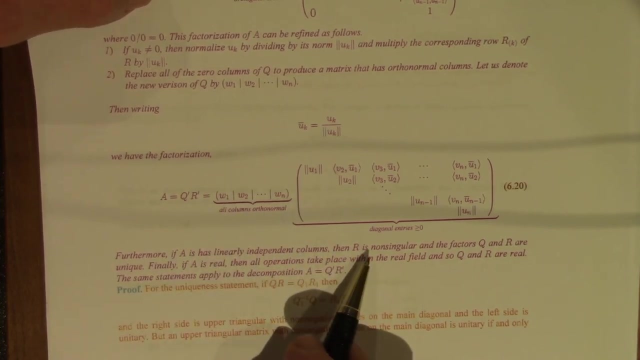 So the QR factorization will be unique. So will the Q'R' factorization. Both of these will be unique. Moreover, if A is a real matrix, all the operations we've done take place in the real field. We didn't have to take any roots. 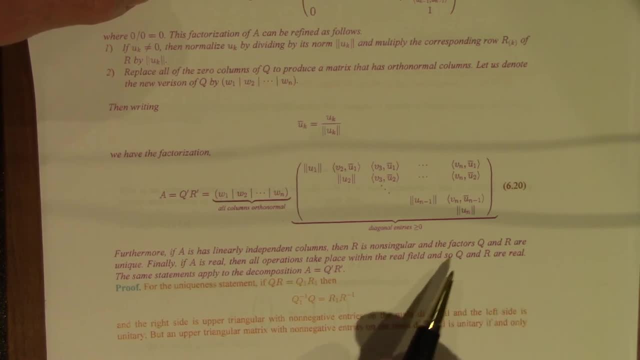 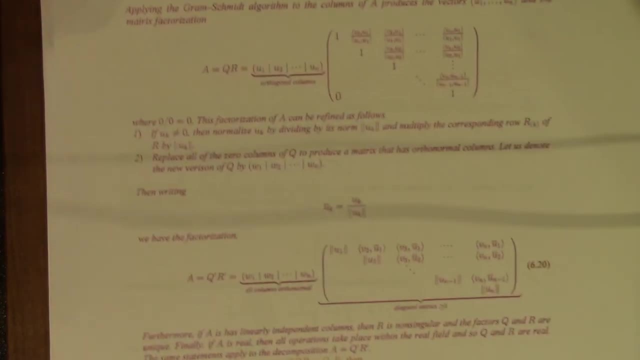 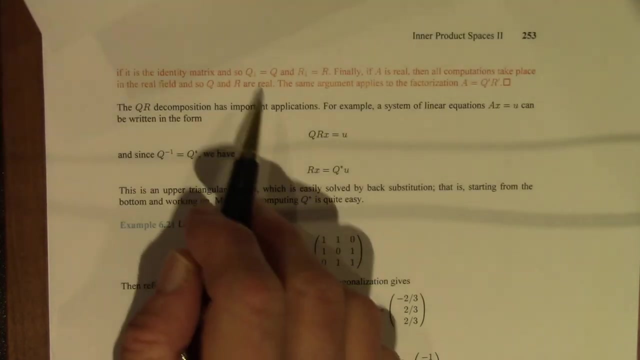 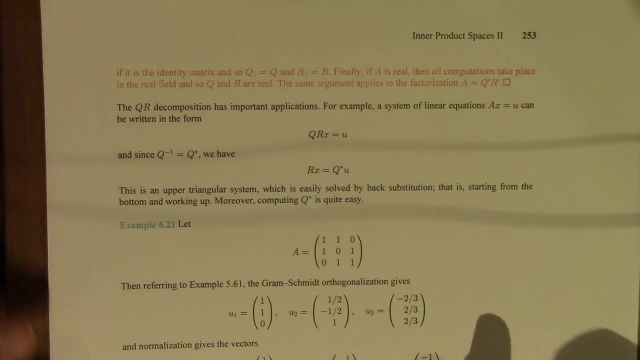 square roots or otherwise, And so Q and R will be real matrices. That works for both forms of the QR factorization, And the uniqueness proof is just one, two, three, four, six lines. So I will let you think on that. 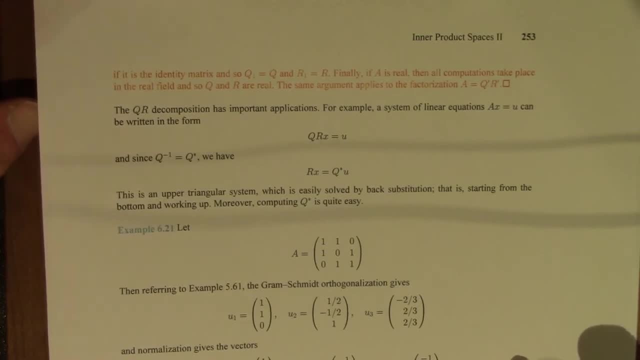 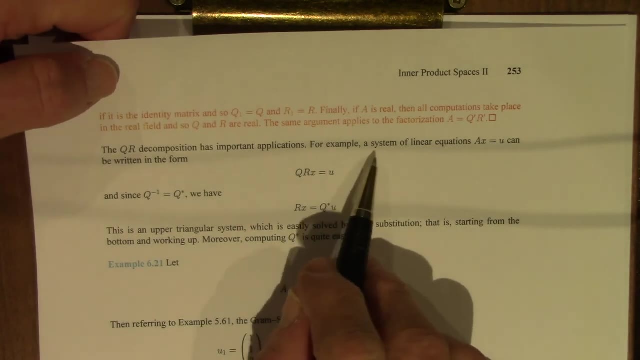 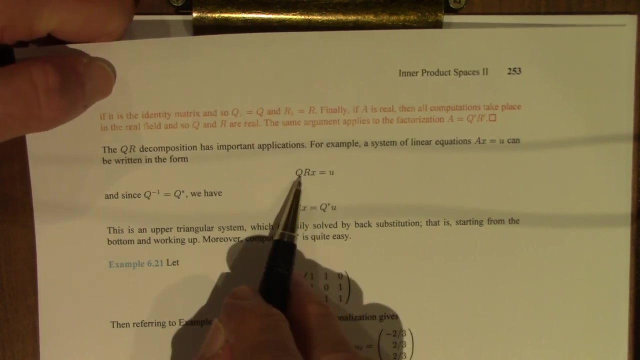 The QR factorization has very important applications. A system of equations AX equals U can then be written in this form: QRX equals U, A is factored in the QR factorization, And when Q has orthonormal columns and when M equals N, 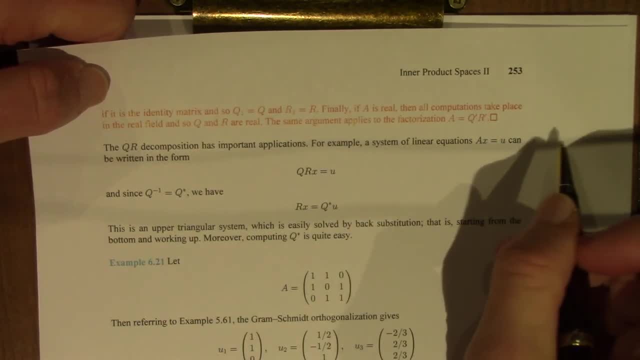 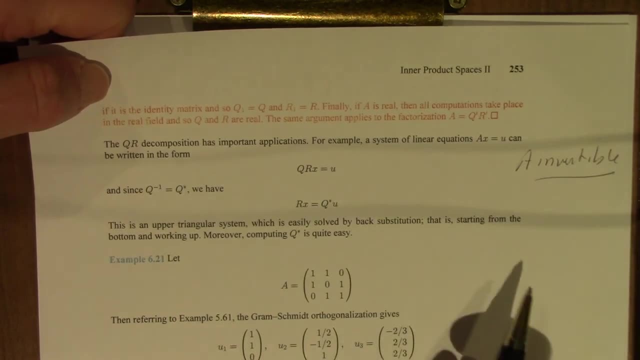 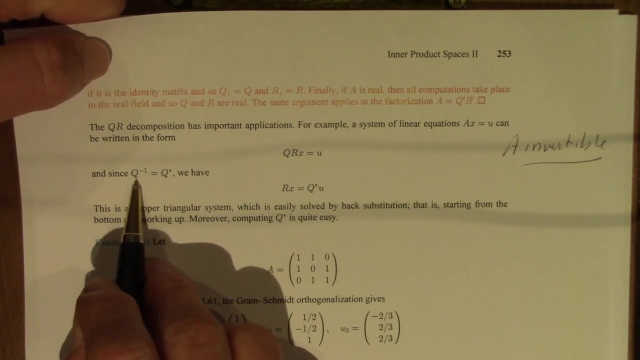 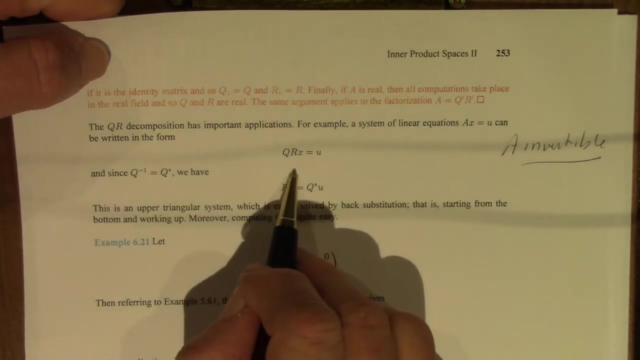 so I should have said all that in here. if A is invertible, that's a better way to say it. I better add that then Q is a unitary matrix, so Q inverse is Q star, So we can move Q to the other side. 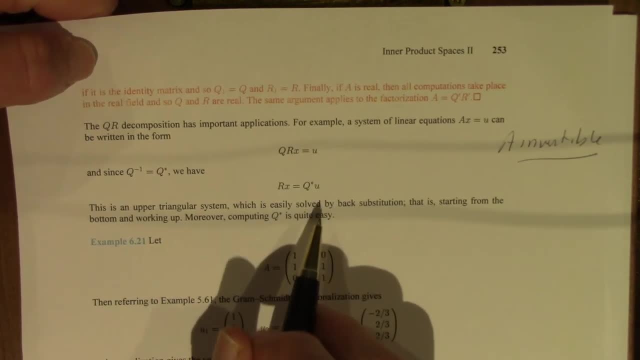 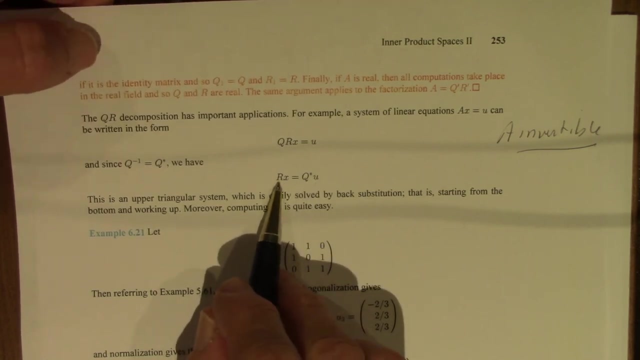 it becomes Q star. Q star is easy to compute from Q it's the conjugate transpose, so it's much easier to compute than the general inverse of an invertible matrix. And this equation- here R is upper triangular, so this system is easy to solve. 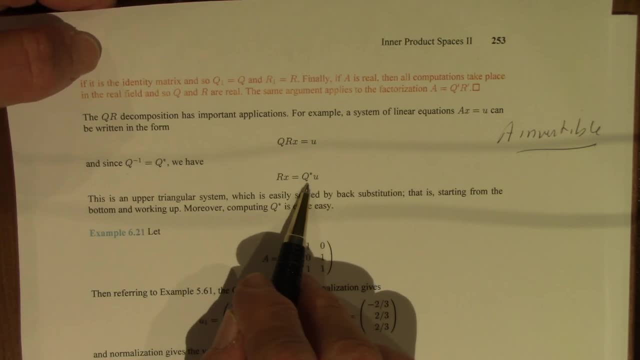 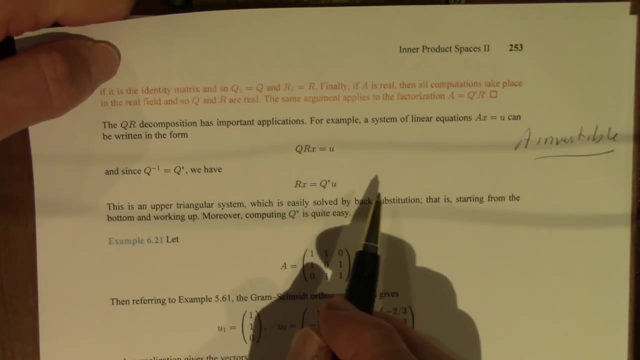 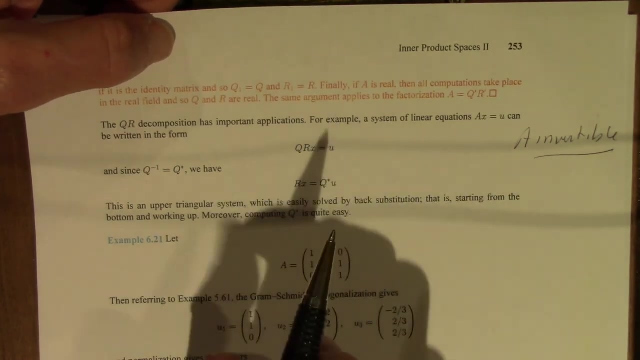 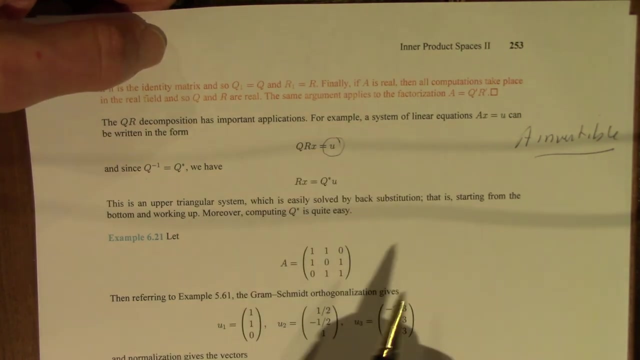 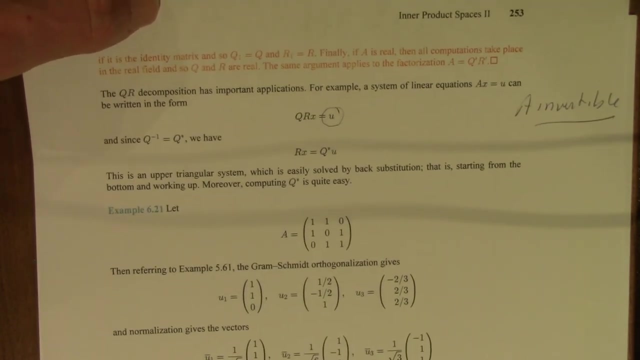 by what is called back substitution. So we start from the bottom and work up. So when you have this QR, factorization of an invertible matrix solving systems of equations- this U can be different values could change- is quite simple. So for example, 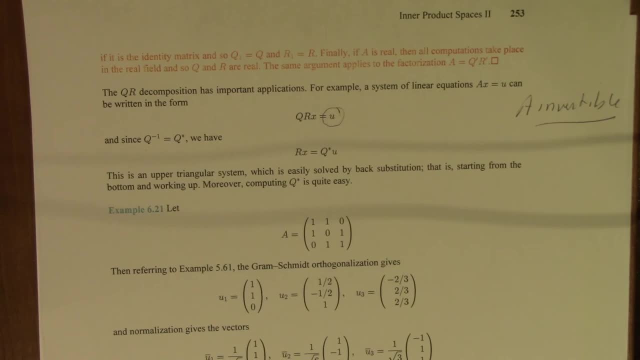 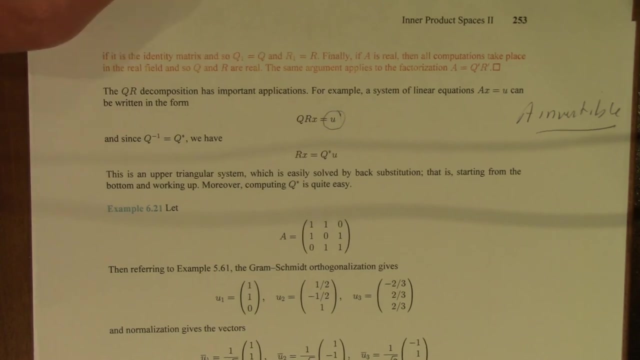 let's say you had a black box that took input and produced output in the form of vectors from FN and you knew that the matrix, the black box, was a matrix multiplication, it was a linear box and that it was invertible. You might have 10,000 outputs. 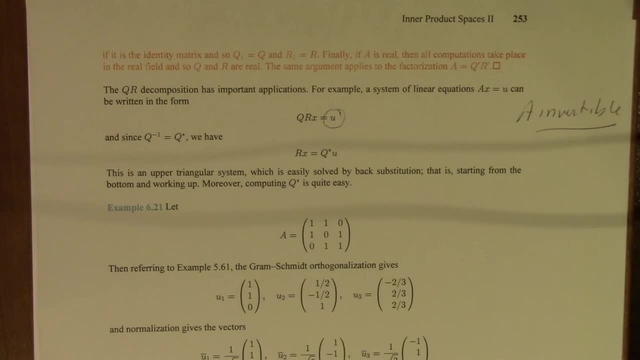 and you might want to know what the inputs were for each of those. So it would be possibly the best procedure would possibly be to find the QR factorization of the matrix A, and then you'd be able to solve these equations very quickly.